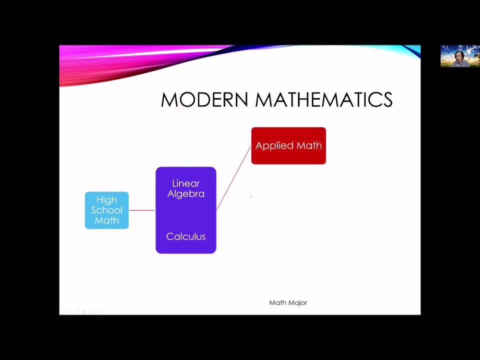 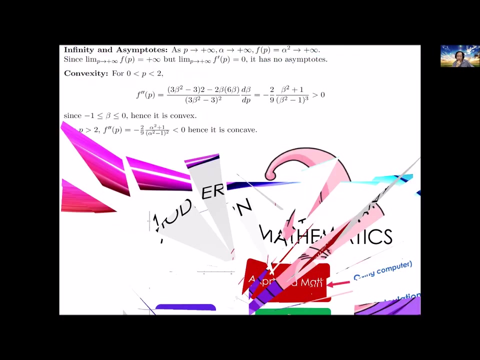 to do the abstract setting. And after this, you will learn to study different kinds of areas in mathematics. So I split out applied math, which is the calculation that really just use computer, and I don't consider those as pure math. For pure math, there are usually three main topics. One is analysis, which is real calculation using pen and paper. And for those students who are in this class, I think you guys all have nice experience to introduction of mathematical analysis already, by doing calculations on 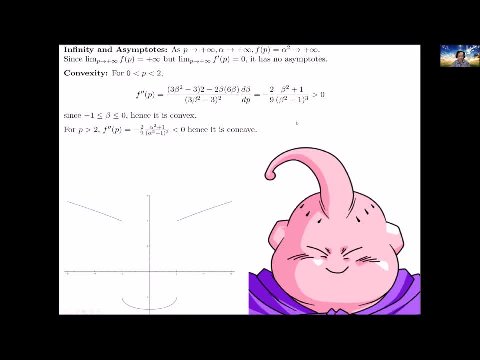 pen and paper, and trying to draw this graph from the final exam. Yes, okay. Nice. 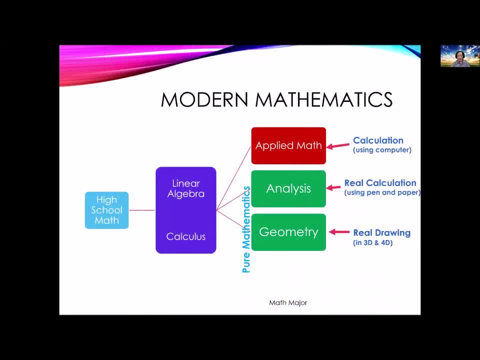 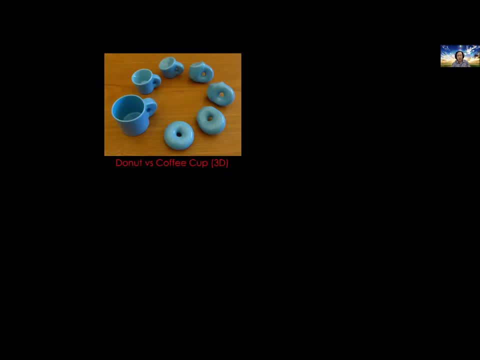 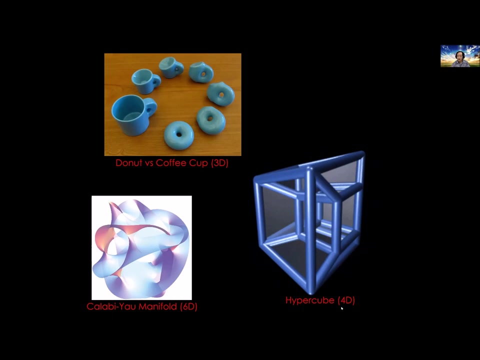 So the next topic is geometry. And this is about drawing. And most of the time nowadays we focus on 3D and 4D. So yeah, coffee cups, like a doughnut is a very famous example. And Calabi-Yau manifold in 6D is a research area in many of our faculties, like Frederick Fong, and so on. And yeah, some nice cool animation I found online, like 4D hypercube. Yeah, Yao is Yao-Sing-Tong, a famous mathematician. Yeah. Yeah, it's so cool. 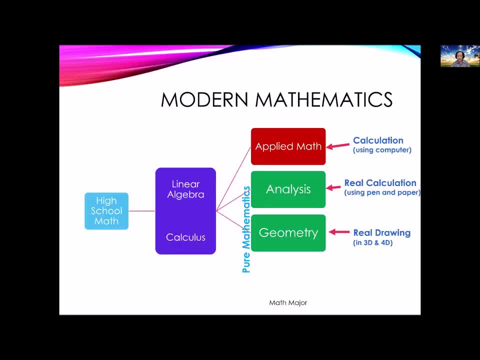 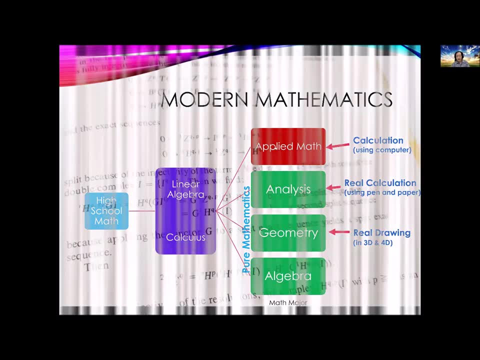 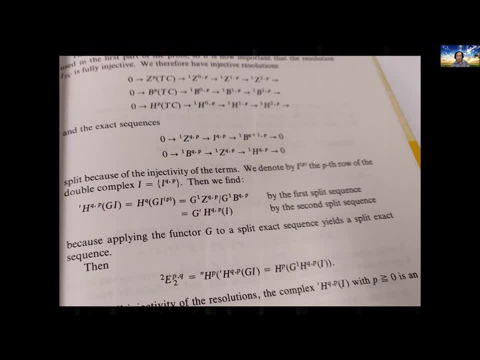 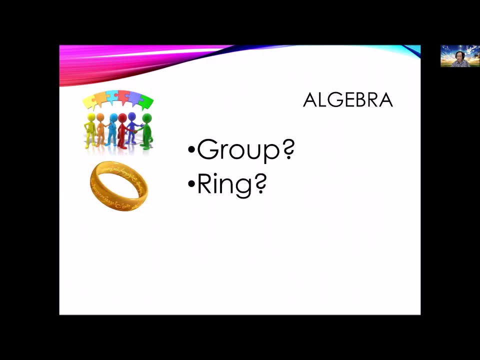 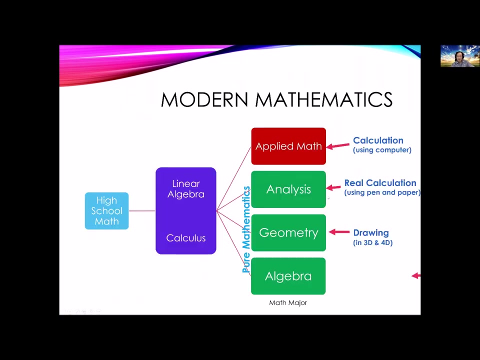 All right, the last topic is algebra, the huge topic, and if you describe any algebra taskbook at once, you will see that things are pretty abstract, and they are all like in symbols, and there names like groups and rings and field and what are all this stuff and why are we going to study this stuff well it turns out I'll talk about where this comes from but it turns out that yeah so real we don't know what's going on but it turns out that a lot of mathematical papers nowadays actually use the language of groups rings and fields and not even in pure math but also in applied math this language will happens everywhere and the main reason is from 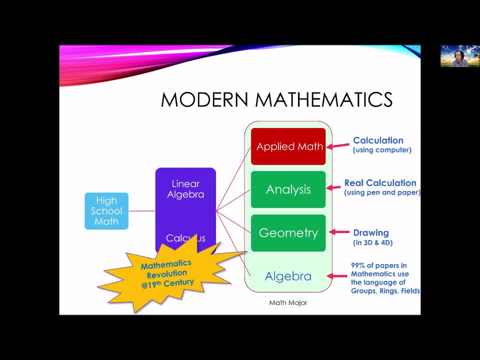 the mathematics revolution in the 19th century about 150 years ago right so to 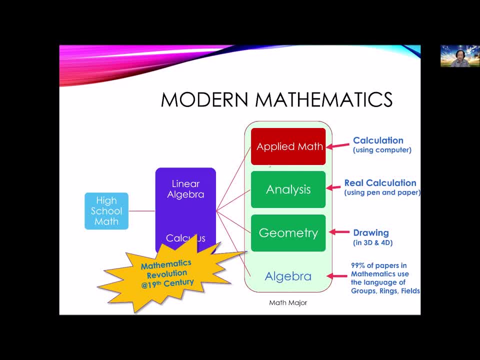 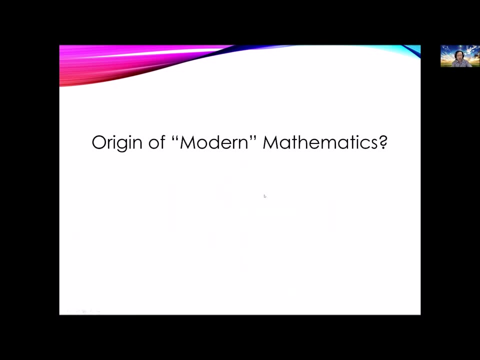 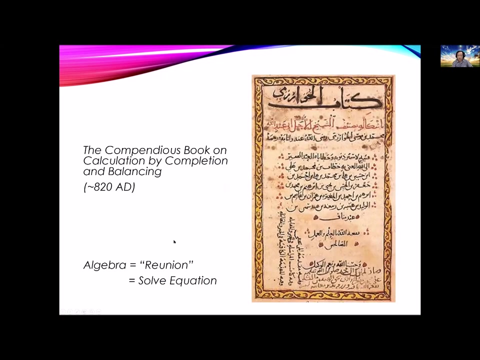 give you like an introduction of this algebraic object so we have to go back to the origin of modern mathematics so what is mathematics what are we trying to do for let's say for the ancient people well of course is to solve equations and the name algebra basically that comes from the elaborate term called algebra yeah which means reunion or in a more elaborate meaning really just to solve equations so that the unknown variables are reunited with this solution. 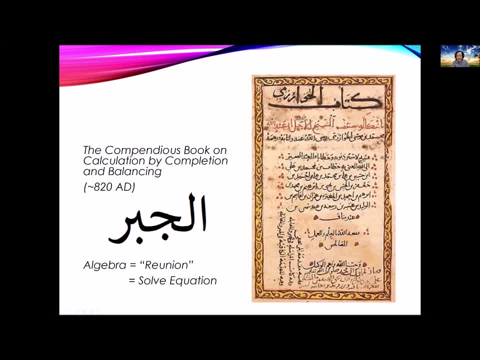 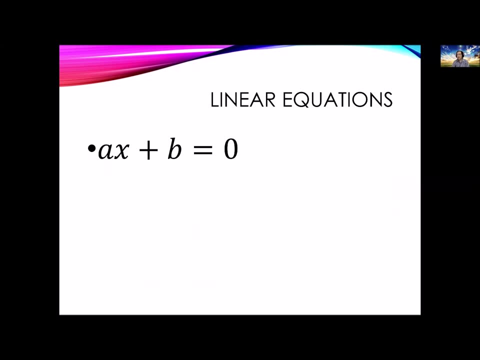 So, I don't know where's the algebra in this picture, but yeah, this is the book, called the Compendious Book on Conversion by Computers and Farmers, or whatever. Yeah, so this is the algebra term. So, what is the simplest equations that one can ask? Well, of course, the linear algebra, linear equation, AX plus B equals zero. And what are the solutions of this equation? Well, there are no solutions, because ancient people do not know how to use negative number. So, instead, yeah, let's do this, 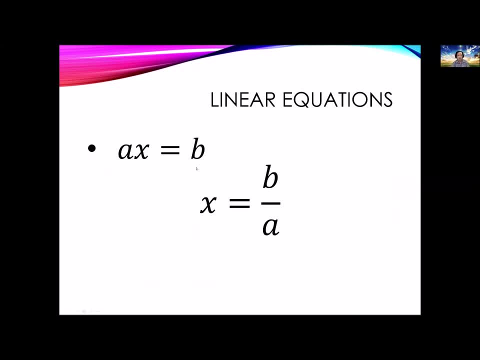 and then ancient people know how to solve this, of course, just by D over A. So, this linear equation, and then the next step will be, of course, quadratic equations. And we all know, learned from high school, that we have this quadratic formula that tells you how to solve this equation. 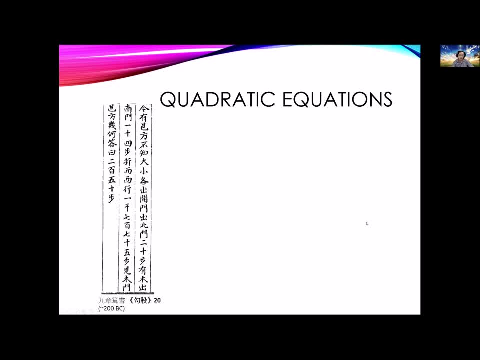 Although this quadratic equation is already known pretty much long, very long time ago, for example, in 200 BC, like 2000 years ago, already we have examples from China in these nine chapters of arithmetics that tells you a problem in quadratic equations. So, just to translate, it says that we have a square city wall that we don't know the size, and if we walk north by 20 steps, we can see a tree. 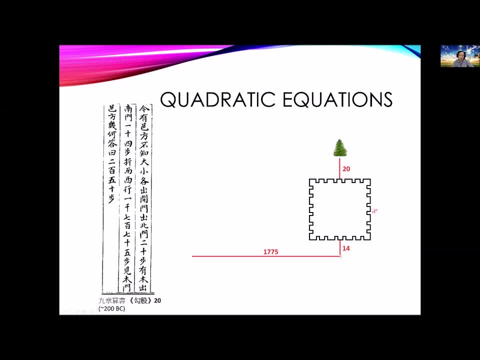 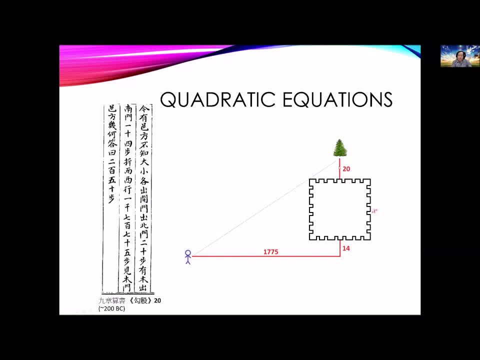 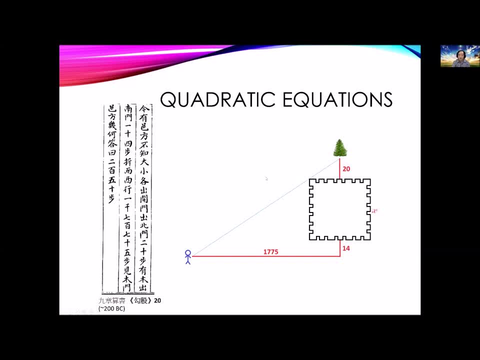 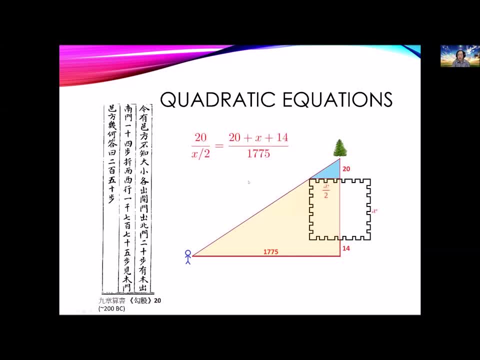 And if we walk south by 14 steps, we can see a tree. And you look at the ratios of the size and the ratios of the height, and you rearrange the term and you will get the quadratic equation. 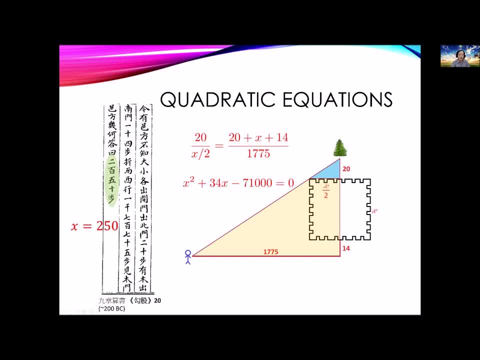 And from this, we can be sure that the ancient know how to solve quadratic equations and get the answer X equals 250. 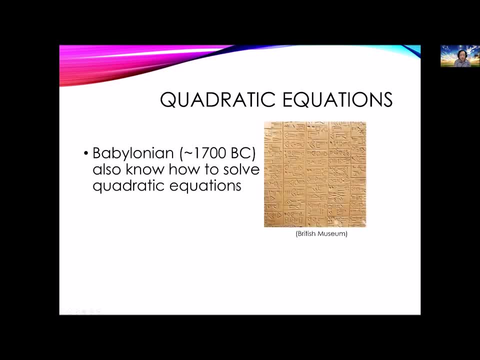 But this is not the oldest known result because the Babylonians actually even know how to solve this equation in 1700 BC. 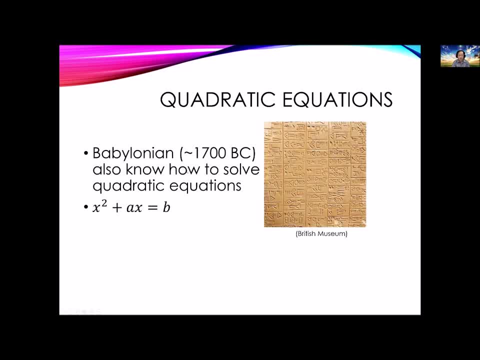 And so this is the record in British museums, although it's more like a special case. So, because as I said, they don't know how to use negative numbers. So this is the special case that they try to solve and they have this answer. And this is also recorded in the same algebra book that I mentioned previously. 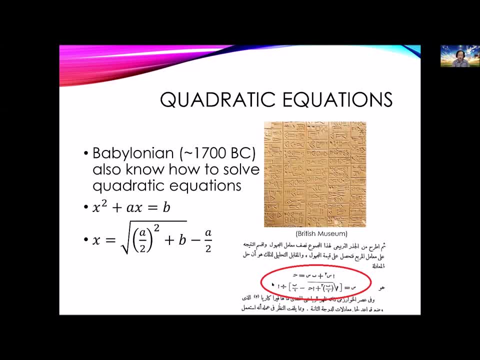 So in Arabic, the writing is from right to left. 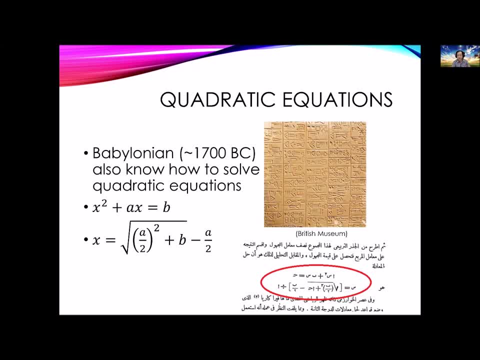 So the symbols are kind of mirror. But you can see that this is the same formula, more or less. 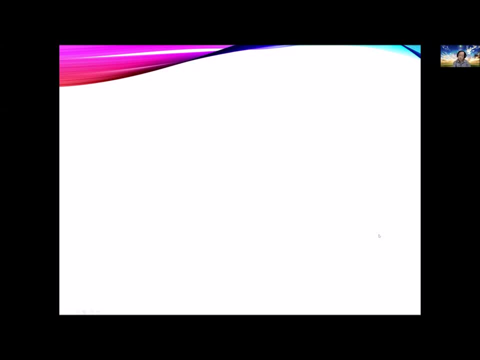 All right, so now we know how to solve quadratic. So how about cubic? 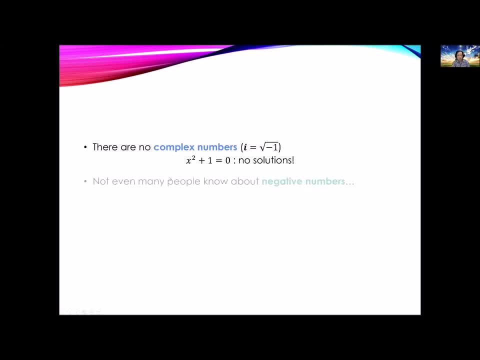 So yeah, at that time, there are no complex numbers, of course, and not even many people know about negative numbers. So, cubic equations is definitely impossible to even think about. 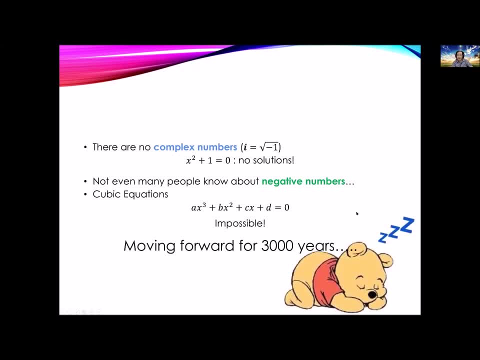 And with this, we have to move forward for 3,000 years after this Babylonian type. 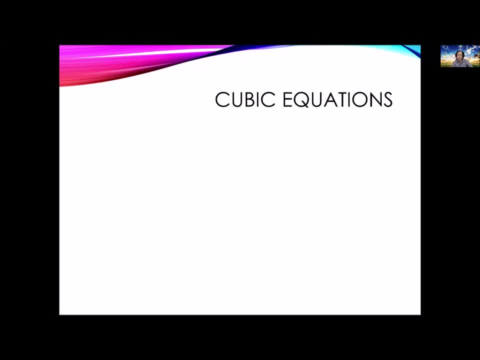 There are no progress at all to solve cubic. Until the Renaissance. 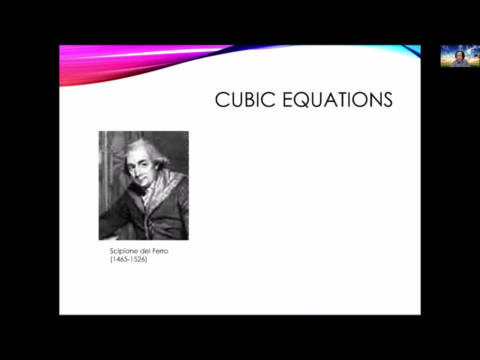 So here comes in the 15th century, a mathematician from University of Bologna. So this is called the Pharaoh. 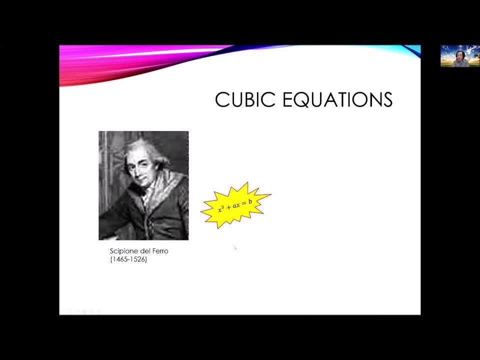 And somehow, after 3,000 years, he knows how to solve a special case of this cubic equation. 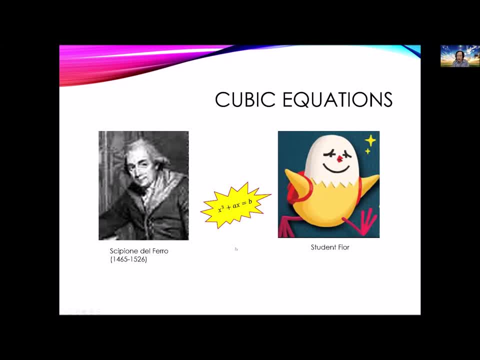 So he has a student, which is called Fyodor, and I cannot find a picture. So I'll just use a seal hot guy to represent him. 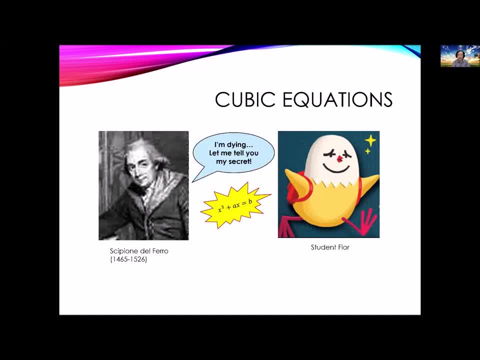 So he's the student of the Pharaoh, and the Pharaoh is dying, and he wants to tell the secret to his student. So at that time, knowing how to solve equation 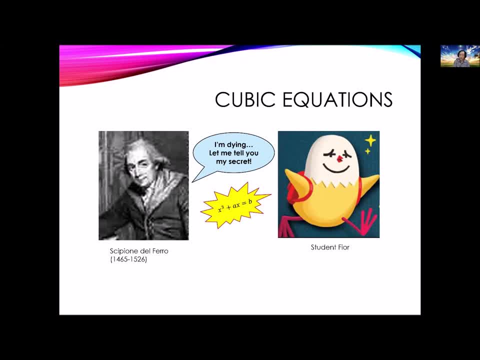 is really a secret weapon or commercial secret, because this is how you raise your fame by challenging other mathematicians. 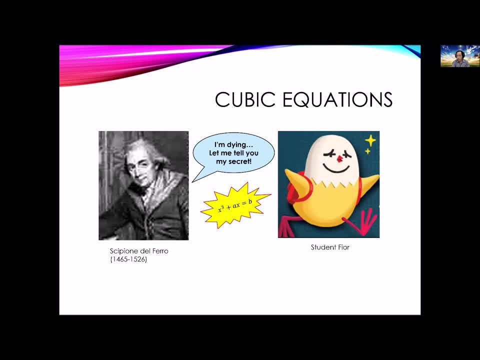 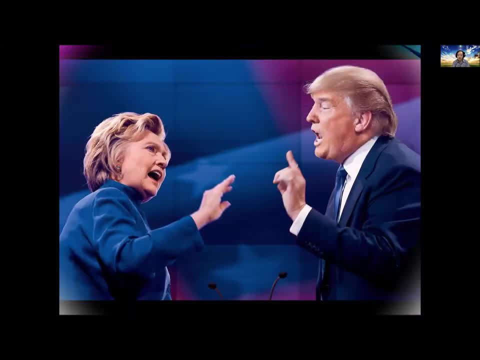 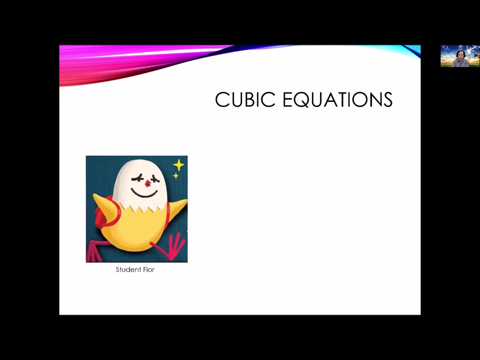 So in this middle age, your reputation as a mathematician is raised by participating in debates or challenges with other mathematicians, just like, yeah, challenge between two people. And actually, there's a very specific format. So each person has to propose 30 problems to the other mathematician, and whoever answered the more questions win. And if he wins, then he'll get more reputation and he may be hired to better jobs and have a better career. 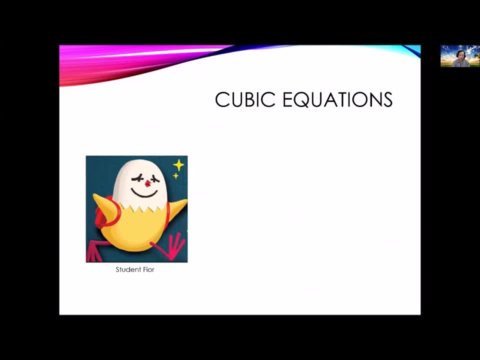 So the student Fyodor, who knows this secret, he wants to challenge a cubic equation solving techniques from his teacher. He start to challenge other people, and he choose Tartaglia, which at the time is a very famous mathematicians from Venice. So he want to challenge Tartaglia, 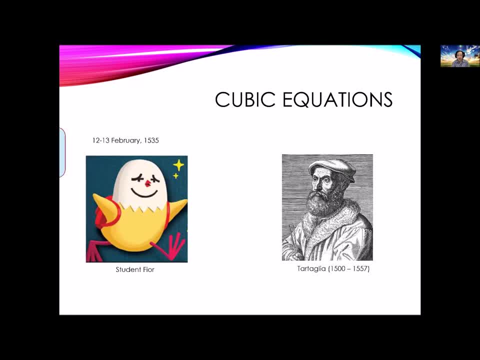 and because with his cubic equation techniques, he asked all 30 questions about solving a cubic equation. And Tartaglia, he's a normal mathematician. 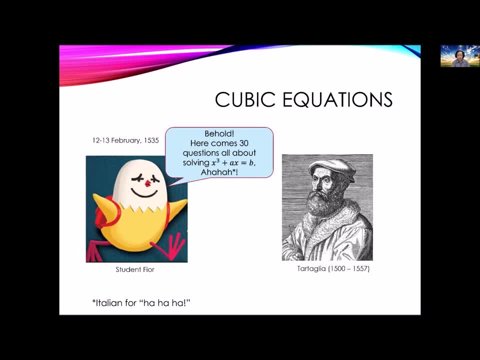 He submit other different variety of questions to the student Fyodor. 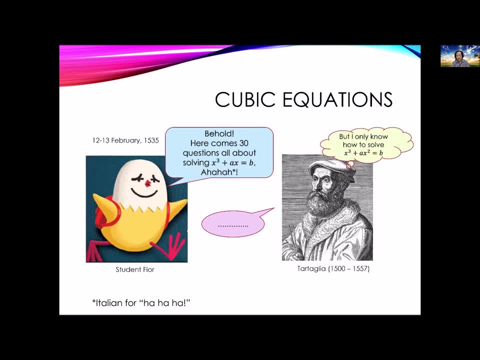 But he's a famous mathematician. So actually he's also a professional and he already know how to solve another special case 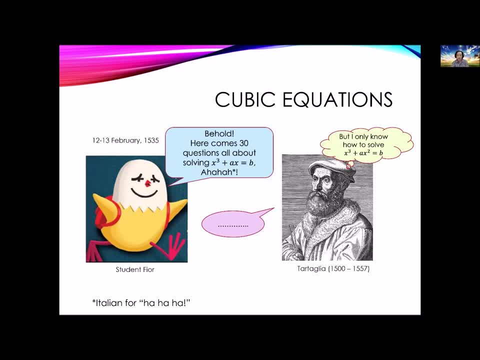 of cubic, SQ plus AX squared equals B, not exactly the same form as the one that Fyodor proposed, but similar enough. 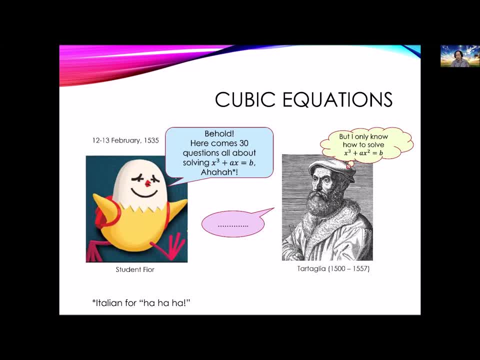 And in our modern days, we definitely know that if you can solve this, you can take one over X, and you will get the answer for the other type of cubic. 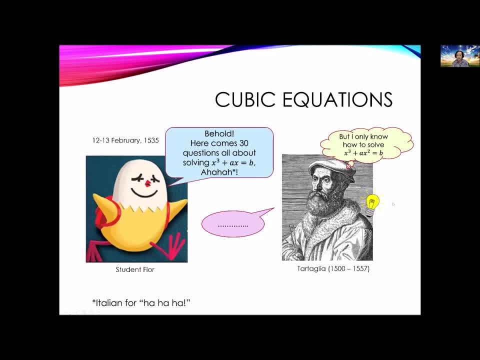 And Tartaglia also realized that. And at that night, 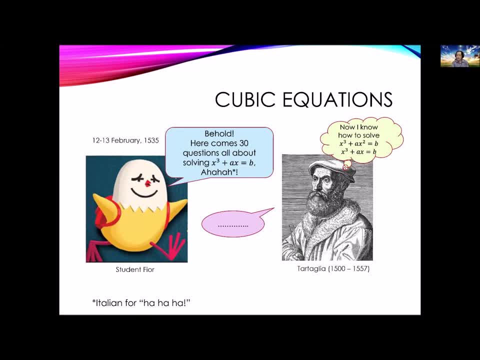 he know how to solve both cases. And he's able to solve all 30 problems of Fyodor in less than two hours and completely defeated him. 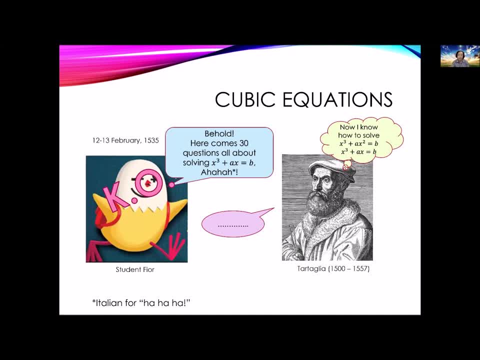 Because I mean, Fyodor asked 30 different variety of problems and yeah, of course he cannot understand, and he can not solve most of them. 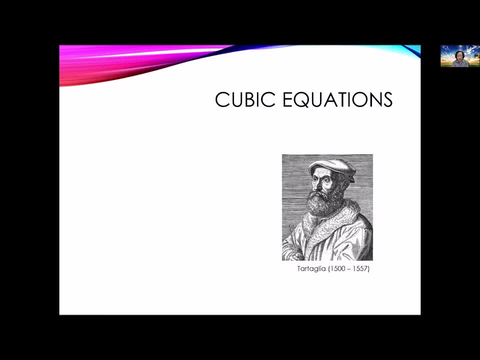 So this public debate turns out to be a news around Italy and a very famous public mathematics lecturer called Cardano heard the news. And he's so intrigued because he's trying to write a book on algebra. And he previously thought that the solutions to the cubic equation is impossible. 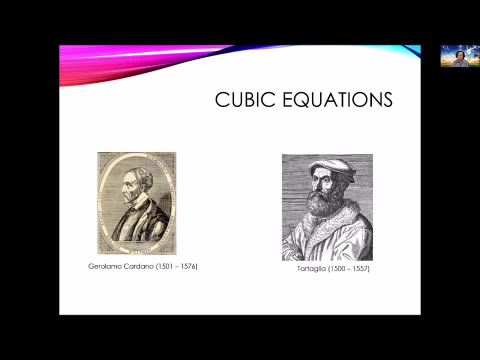 And now he learned about this public debate and he learned about the fact that, that the cubic actually can be solved, he wanted to include this solution to his new book. 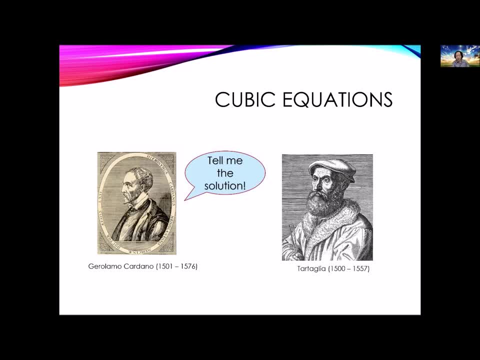 So he found Tartaglia and asked him to provide the solution. But of course, this is a commercial secret, as I mentioned last time, and Tartaglia still wants to use this solution to beat maybe other mathematicians or just to be secure for his debate. So this debate continued for nearly four years. I'm just speaking like that. Until the publisher, the Cartano, 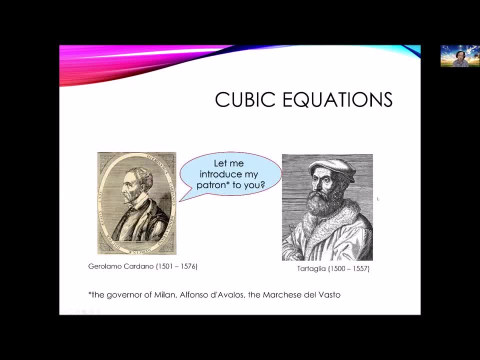 persuade Tartaglia by introducing him to his patron, which at that time is the governor of Milan. So if the governor knows you, then you, I mean, you'll get basically just better jobs and better salary and so on. So finally, Tartaglia accepted his offer. 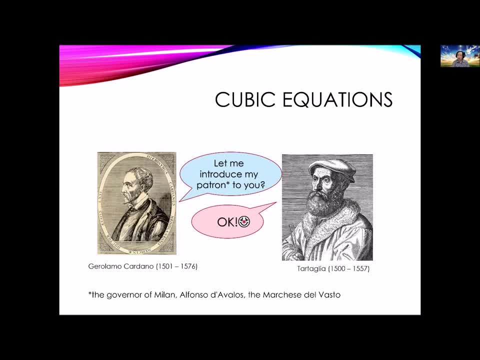 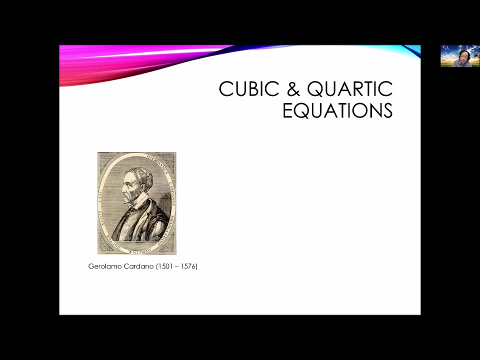 And provide the solution to Cardano in the form of a poem in 1539. And he asked Cardano to never, never publish his solution. Because as I said, this is, should be a commercial secret. So now Cardano equipped with his solution he quickly collaborate with his student Ferrari, I mean Ferrari, and construct the solutions to general cubic, not just the special case that Tardaglia know, but more impressively, not just cubic, but they actually can generalize the solution to quartic as well. So using just Tardaglia's method, they are finally able to solve both the cubic and quartic degree four polynomials. 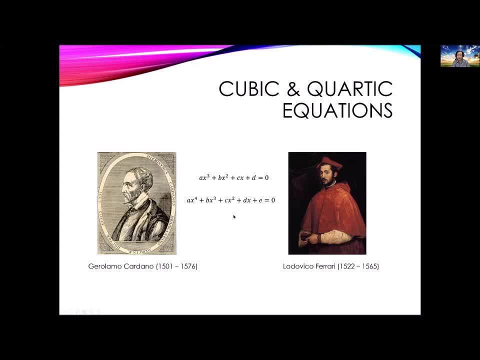 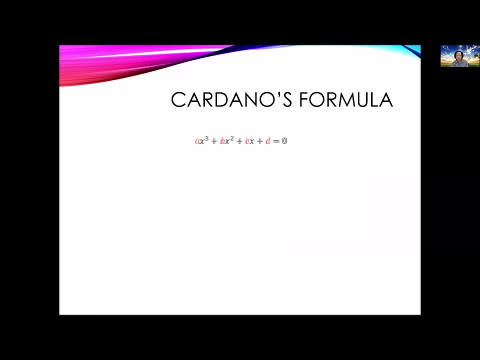 So just to give a more mathematical setup overview, what is the Cardano's formula? It's actually quite easy to understand. So you start with a cubic, and of course you can always normalize by dividing by a. So you have a polynomial that has leading term x cubed only, and we do a simple substitution, and with this we can remove the a from the x squared term. So this p and q will be the original a and b. 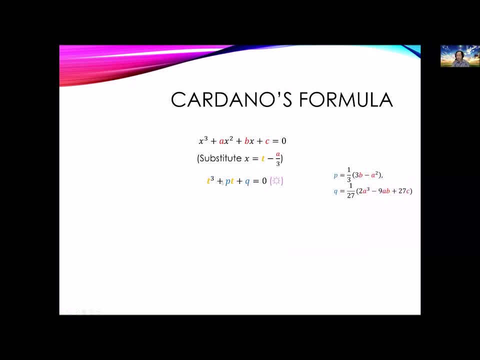 So now you reduce your equation to a cubic where you don't have the x squared term. 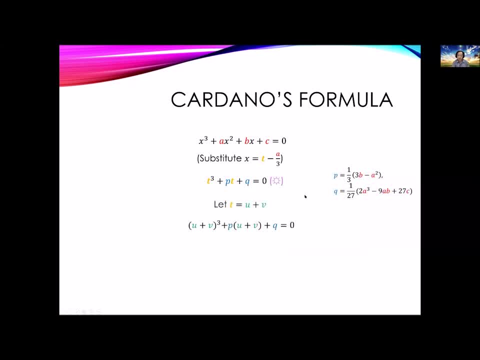 And now you do another substitution like this, and do a rearrangement. 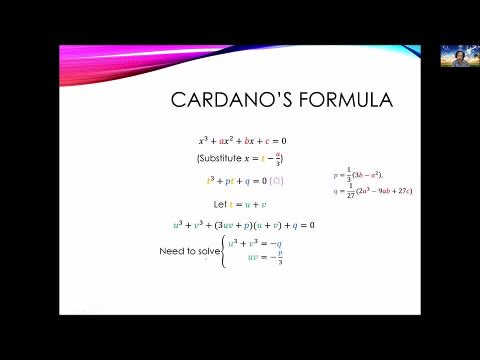 So the idea is that we want to solve this u cubed plus v cubed equals minus q, and free uv plus p equals zero. So if you can simultaneously solve these two equations, then of course this equation is satisfied, right, because you have two times equal zero. 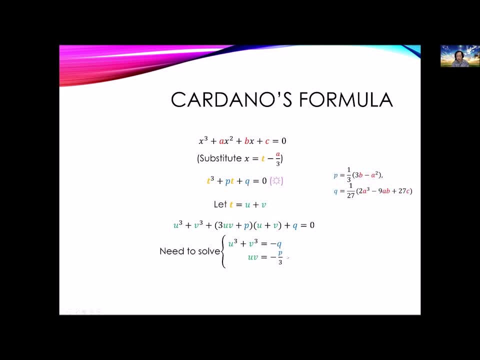 But this equation is satisfied, right, because you have two times equal zero. So for the auxiliary equations, you can modify a little bit by taking a cube. 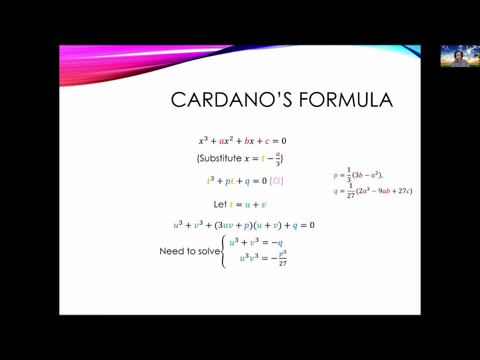 So everyone should now recognize what is this. This is really just the sum of root and product of root, right, if you let alpha equals u cubed and beta equals u cubed. And sum of root and product of root are definitely just quadratic equations, and everyone knows how to solve quadratic equations. So the idea is if you solve the quadratic equation, which is called the Resolvent equation, like this, and you solve the quadratic equation, which is called the Resolvent equation, like this, and you solve the quadratic equation, which is called the Resolvent equation, like this, then you found alpha and beta, then you found u and v, then you found t, which is the solution of your original cubic. And so this is the root of your equation, and the other two are just a slight modification if you want. 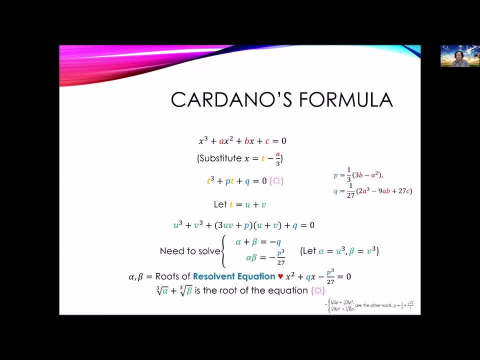 So one can also write down explicitly what this solution in terms of a, b, c, and 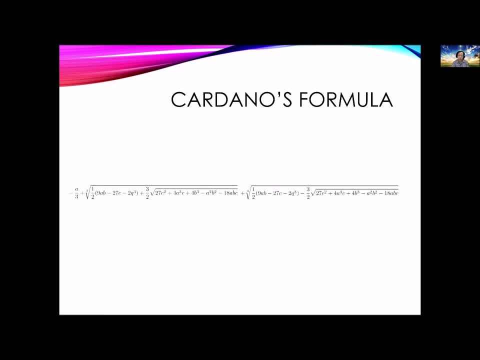 not that bad, not quite long, but not that bad. So this will be the general solution. 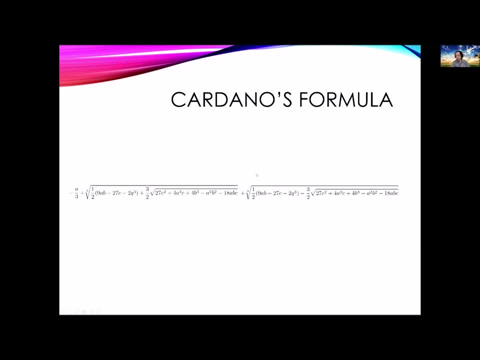 One root of your cubic equation, and this is called the Cardano's formula. 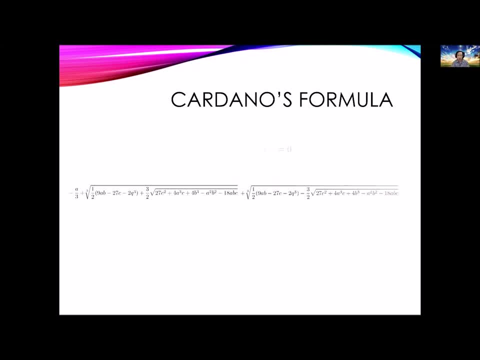 So one can also write down explicitly what this solution in terms of a, b, c, and not that bad. So this will be the general solution. Now, how about the quadratic? Well, the idea is more or less similar. So you have a quadratic, you normalize, and then you do a substitution to remove the first x cubed term, 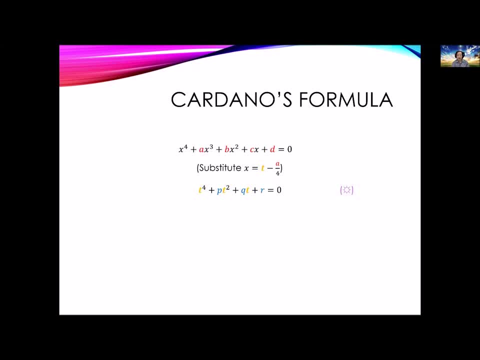 like this, and this time you also have some kind of Resolvent equation, but not quadratic this time. It is a cubic Resolvent equation constructed out of the sum modification of this quadratic. But we already know how to solve cubic from the previous strategy, right? So now from quadratic, we have the Resolvent equation in cubic, and we know how to solve them. So we plug it in, and then we do this modification, and we found that the roots of the quadratic equations are given by plus or minus this expression. So there are three plus or minus, but there are only like four different roots. 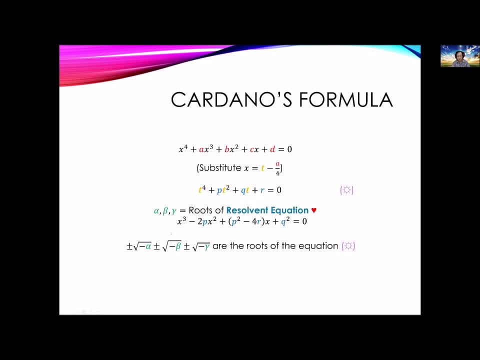 So this will be your original, this will be the solution of your modified quadratic. And to write down the original solution, you can use Mathematica, I think, 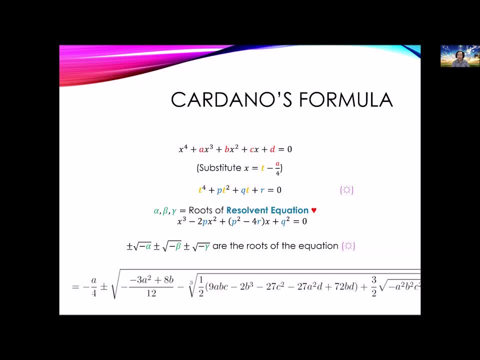 to get the general solution for a quadratic polynomial. I like this. Let me show one more time. 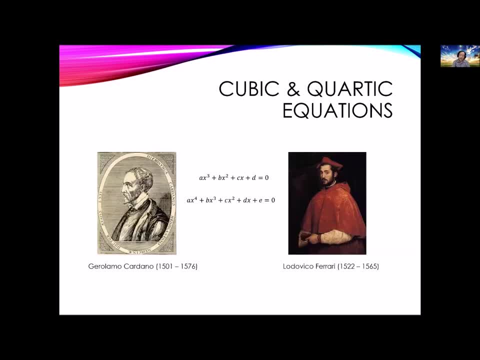 All right. Okay. So now the two guys know how to solve both cubic and quadratic. And as I said, Cardano really wants to write a book on algebra, 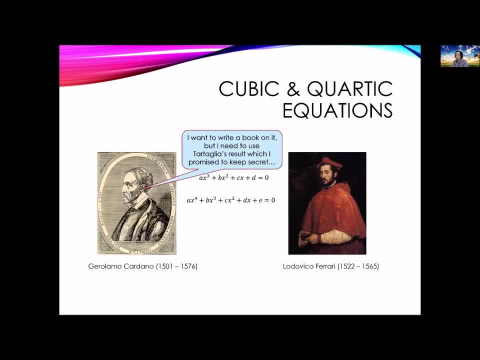 but because he promised Taccardia to keep the secret of his solution. So both formulas need to use Taccardia's method. So in some sense, he cannot publish the book. But in a trip to Bologna, they ultimately found that their Pharaoh, the very first Italian 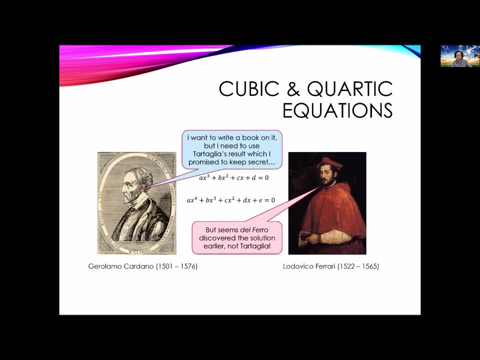 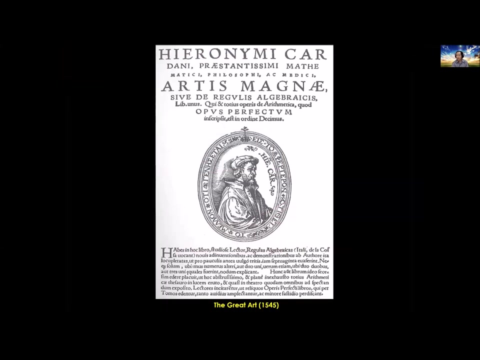 mathematician that I mentioned in the beginning, actually discovered the solutions earlier, not Taccardia. And Cardano is very happy because, I mean, now he has no obligation to keep Taccardia's secret because this secret's not Taccardia's, but really their Pharaoh's. So he published this very famous work called the Great Art and established Cardano as a very world-leading mathematician. 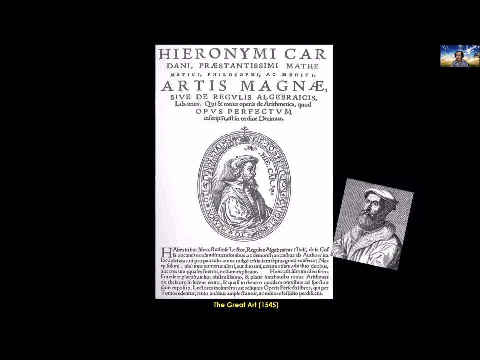 But, of course, Tartaglia, hearing this news, was very furious, and he offered a challenge to Cardano. 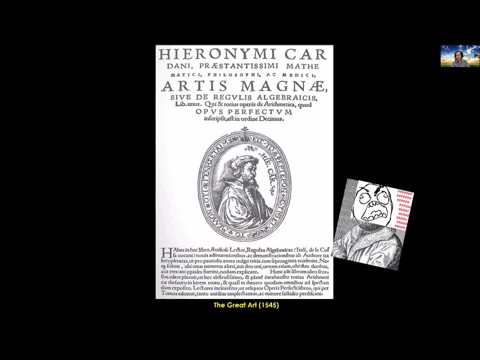 And Cardano, which is now very famous because of this book, of course refused this challenge. And at the end, in 1548, he asked his assistant, Ferrari, to talk up the challenge. And the debate is just one-sided, because Ferrari clearly understood the cubic and quartet more thoroughly than Tartaglia. 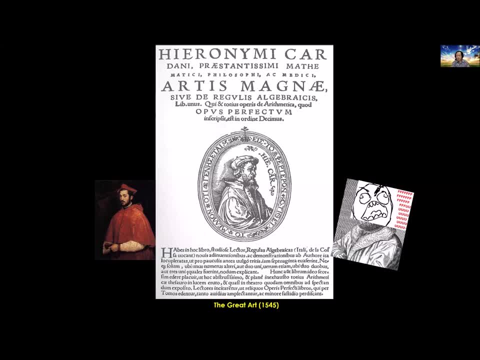 So this debate actually destroyed Tartaglia, and he was later fired from his lecturer job in his hometown, and a few years later just died in poverty in Venice. So it's a very tough time for mathematicians in the Middle Ages, and it is a sad story for Tartaglia, who discovered the cubic, but ultimately was destroyed by his homework. 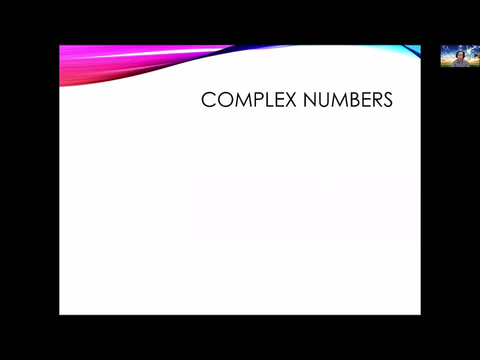 So this story also leads to the birth of complex numbers. And this is discovered by Bombardier. He was a professor at the University of California in the 16th century. 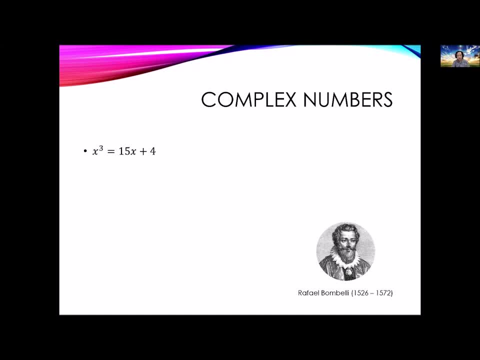 So he looked at this cubic equation, x cubed equals 15x plus 4. So this is just a normal standard cubic equation. So and you can easily check that x equals 4 is a solution, both sides equals 64. But if you use Cardano's formula, the one that I wrote previously, you will see that there are square root minus 121 involved in this solution. And it does. 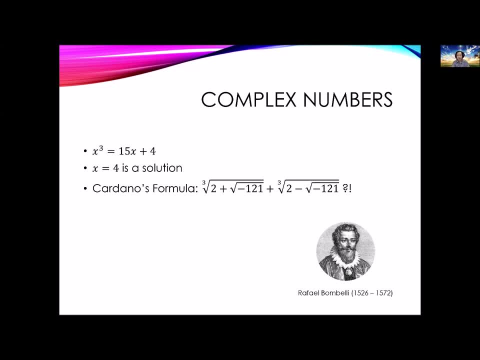 It doesn't make sense at all at the time. So what can he do about that? 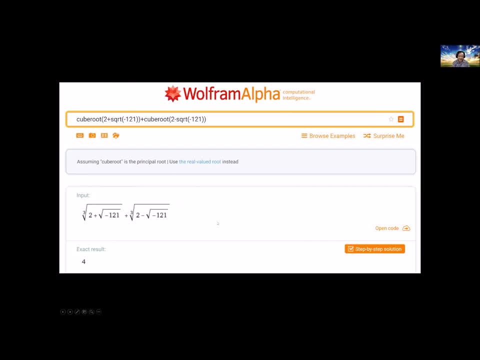 Well, you plug into Mathematica and get the exact result, right? So this is not what Bombardier did, but ultimately he developed the machinery to deal with this square root of negative numbers. 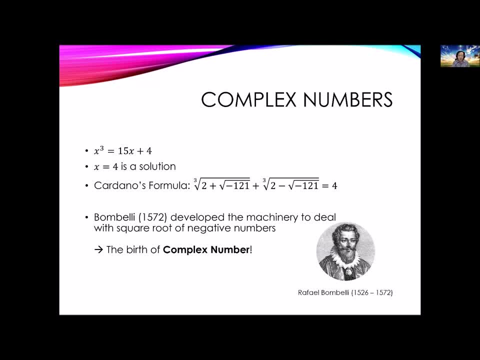 And this is precisely the birth of the complex numbers. So complex number was not constructed out of this x squared plus one solution. But instead, it is discovered because of the problem of applying Cardano's formula to cubic. 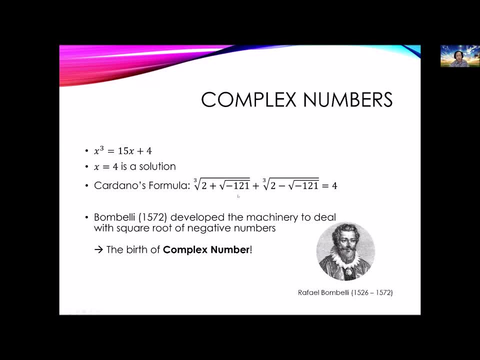 Because this formula always, most of the time, will involve negative square root. 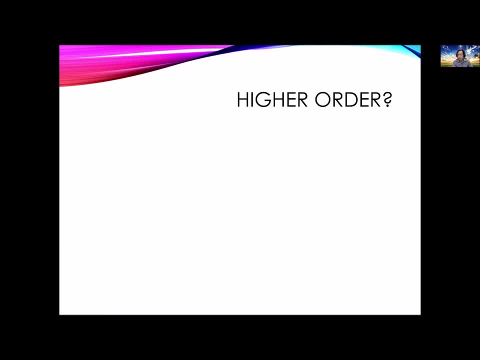 Okay, so that's the story up to degree four. 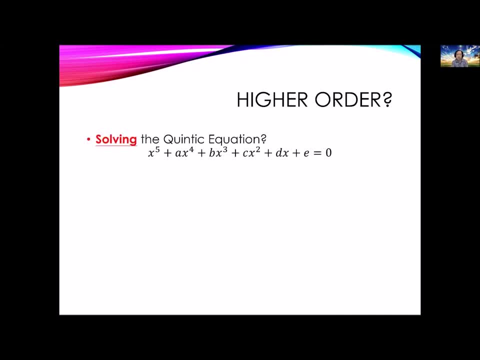 But then, oh sorry, but then what about higher order? So how can we solve Quintet equation? 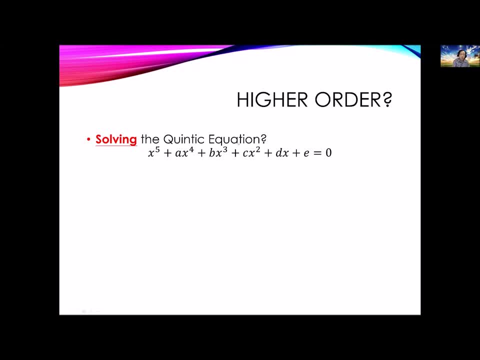 So can we solve equation of degree five or even more? So solving here means that you can only use. Standard arithmetic plus minus, multiply, divide, and possibly taking radicals, taking 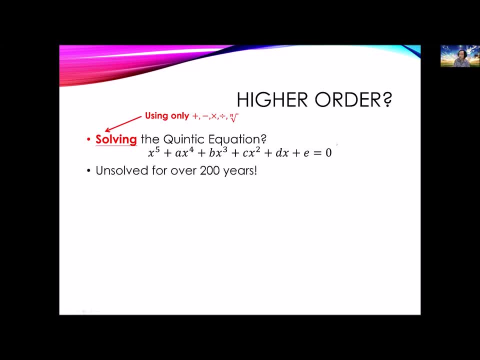 nth roots. So this problem remains unsolved for 200 years. 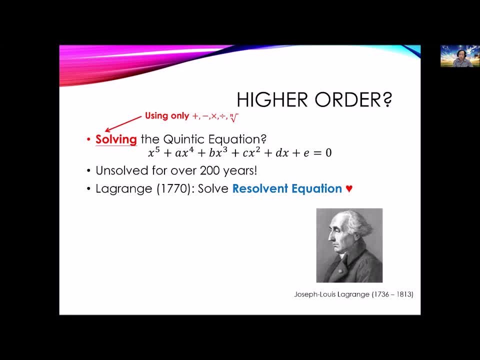 And everyone knows kind of the idea that in order to solve such equation, you want to translate just like the cubic and quartic to some kind of resolvent equation. 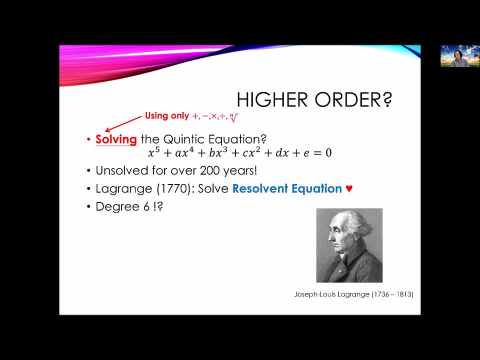 But but for the Quintet, it turns out the resolvent equation has degree six. So it's even worse than the original problem. 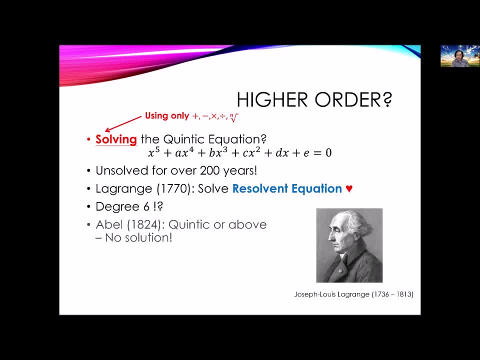 And it is not helpful at all. So the first, the first mathematicians who answered this question is Abel in 1824. 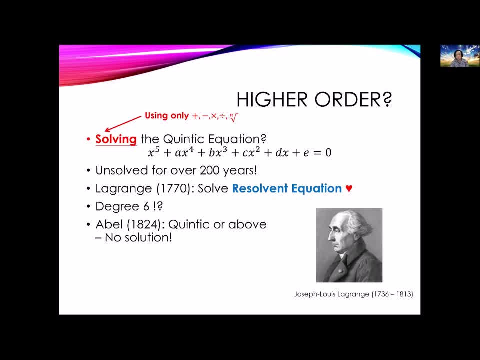 And he concluded that the Quintet or Abel has no solution in terms of arithmetic and taking root. 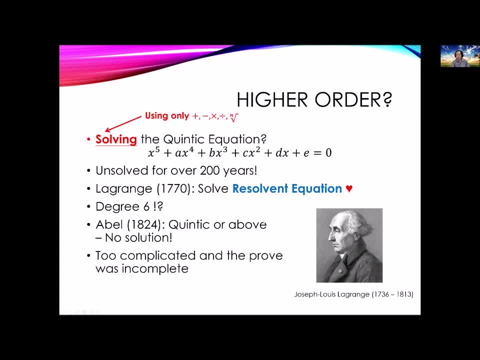 However, his approach is very complicated. 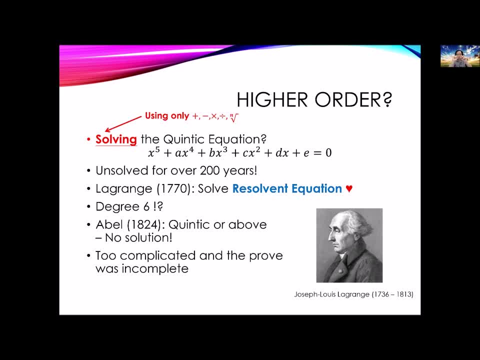 It's like a case by case study of different polynomials with different coefficients. And it was too complicated and it's always thought to be incomplete. 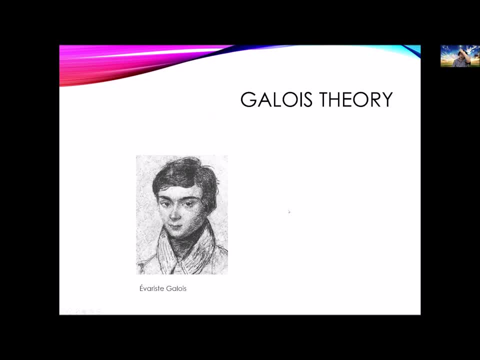 So at last a very smart genius shows up, which is Gawal. So many of you may have heard of his name. So Gawal observed that the resolvent equation is too complicated and he should, we should be working instead on the symmetries of the roots. So he proposed this observation in the last days of his life. 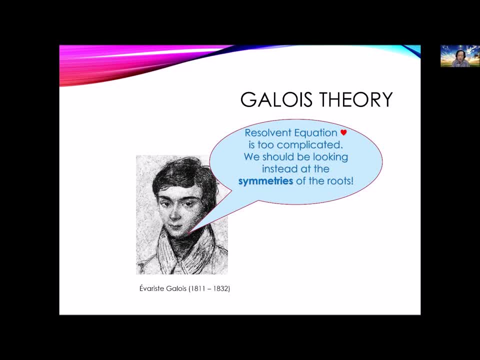 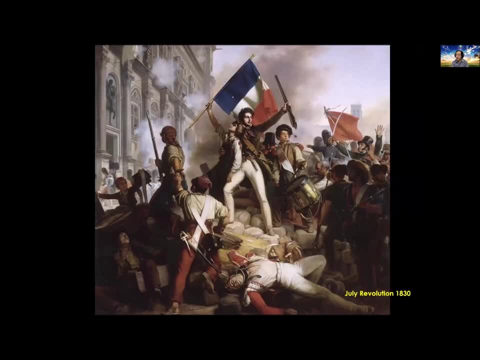 And he has a short life, which is only like 21 year old. So this was the time during the July revolution. And Gawal was frequently arrested from political activities. And for those who are interested, this revolution ultimately led to the Paris rebellion in the Miserra, the Hugo's novel, Miserra, two years later. 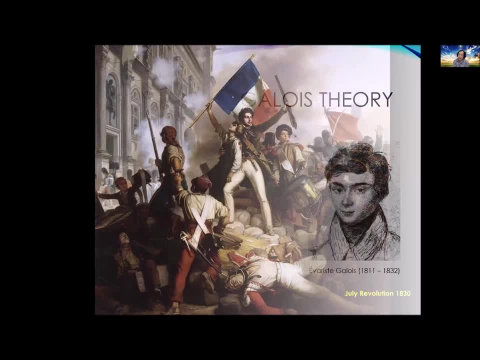 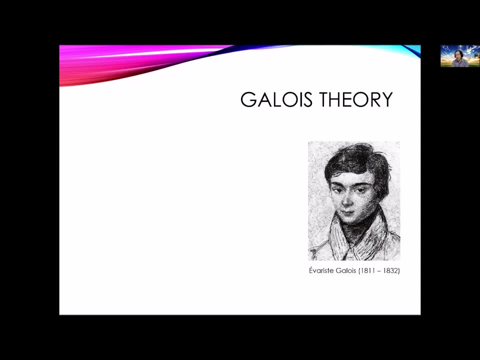 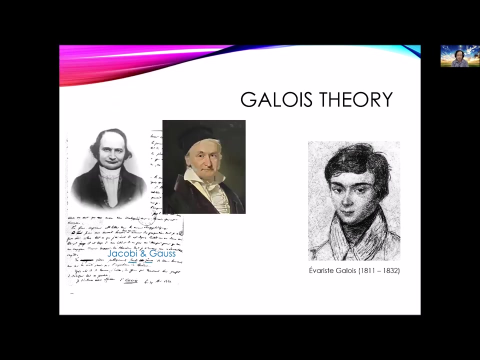 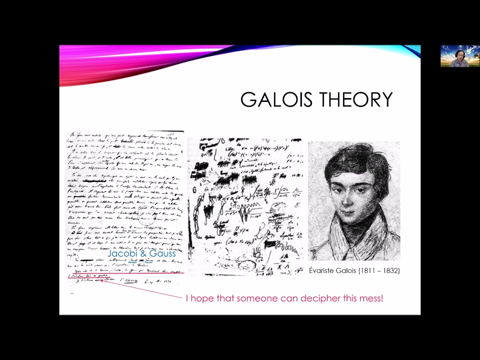 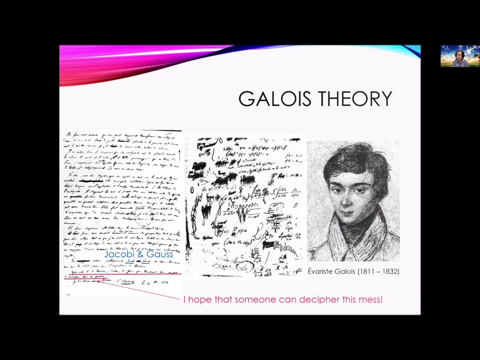 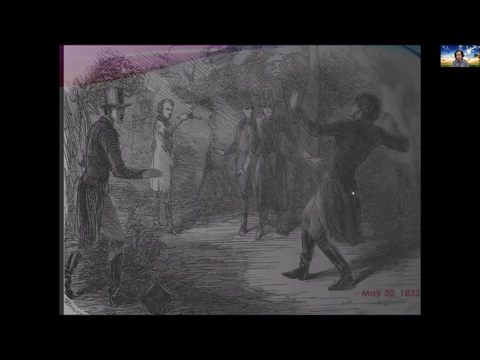 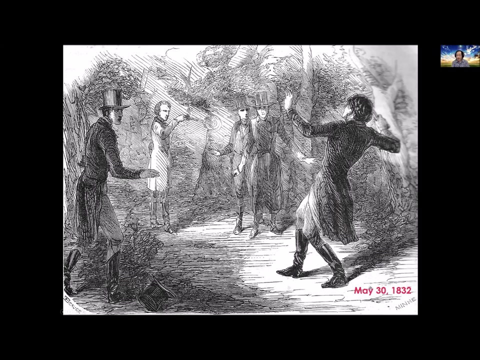 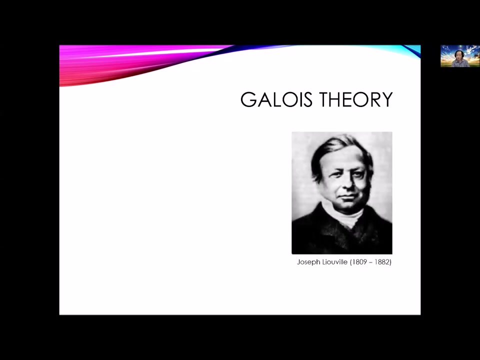 And one day, finally, he was arrested and he has to arrange a duel with a person called Perchaud de Bromfield, which is a rival in politics. So he arranged a duel with him, and he himself know that he probably will not win the duel. So he spent the last days of his life, scraping down all his mathematical works so far and send it to his friend hopefully to bring his work to the two famous mathematicians Jacobi and Gauss at that time so these two guys and you can see from his writing that he just hopes someone can decipher all his mathematical achievement or work so this another part of his script I'm not sure how Jacobi and Gauss will read this kind of script but at the end he fought the duel and just as I said he died at the age of 21 because he just got shot and not cured so his theory was ultimately not read by Jacobi and Gauss but luckily 10 years later a mathematician called Leofield found his paperwork and collect them and make a publication and he was able to do it 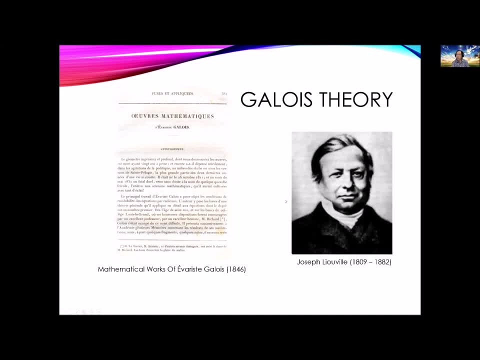 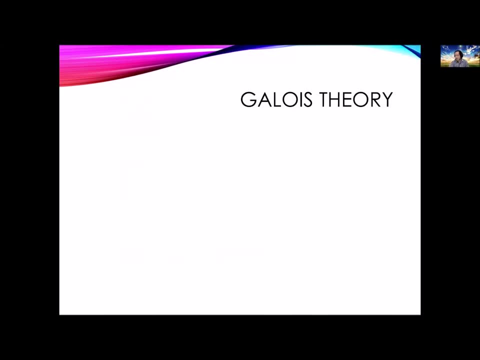 on the work of Gauss so after that everyone knows of Gauss achievement so what is Gauss theory in a very layman term so we have looked at quadratic equation and we know the solution 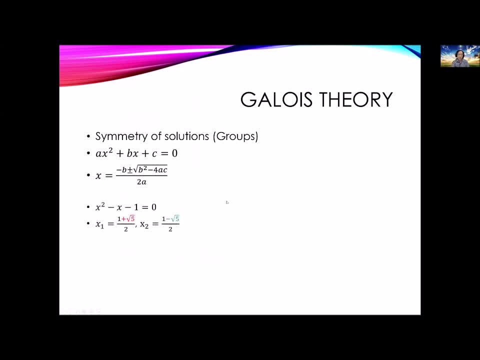 of quadratic equation which is some kind of plus minus square root thing so as an example this x squared minus x minus one gives you a golden ratio and we see that the two roots are kind of symmetric with plus square root five and minus square root five so it's like playing two balls where you can switch the position around and the arithmetic involving the square root five has this symmetry right if you do this calculation with square root five and you just replace plus square five by minus square root five everything still works I mean the arithmetic still is still the same so the things does not change if you I mean the arithmetic is still the same so the things does not change if you I mean the arithmetic does not change if you switch the two roots and this is the first observation of symmetry for cubic equation you have similar thing because if you have the free roots alpha beta and gamma you can always switch the position of this root and your equation will not change so this like is symmetry of three balls by permuting three different objects and another point of view for example C which is the product of roots alpha beta gamma will not change even if you and I permit the position of these roots so Garазд idea is that every equation every polynomial occasions you have a corresponding symmetric groups and for quantic you have similar observations you have a s4 symmetry group which is the permutation of four objects and similarly 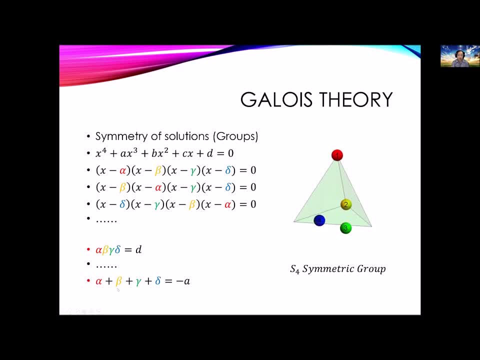 you have observe this coefficient twenty-five times a solution you have incrementally relation A, B, C, D are all unchanged if you just permute this root. 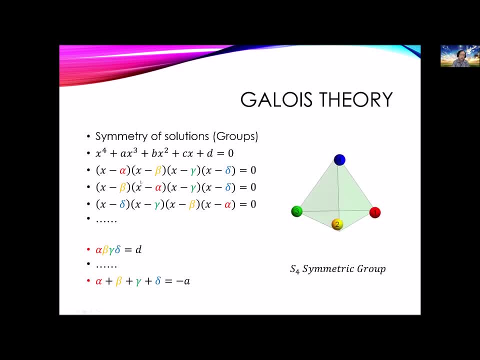 So instead of studying resolvent equations or those kinds of things, 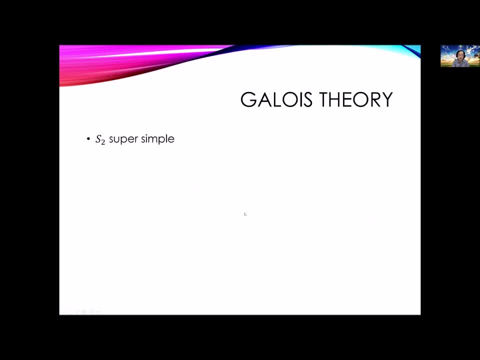 Garval's idea is to study the symmetry of the groups. So we have seen that S2, the one that permute only two things is very simple. S3 is also simple. S4, okay, there's a four board. 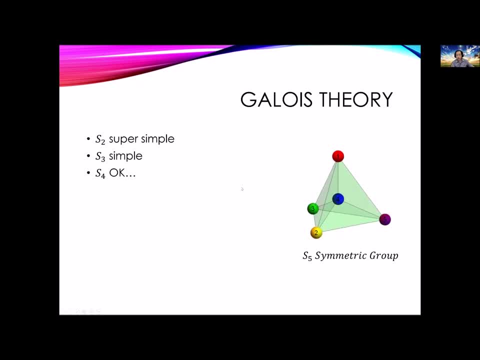 But for S5, I cannot really draw a 4D pyramid. So this is the best I can do. For S5, it is just too complicated. 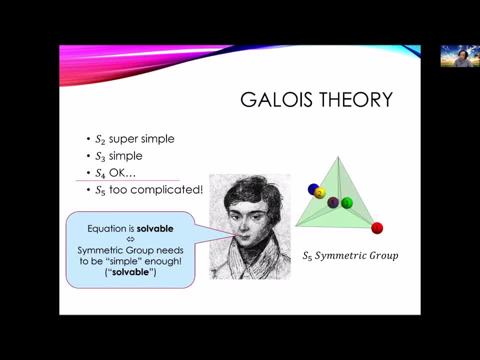 And Garval's observation is that the equation is solvable, meaning that you can solve it in terms of plus minus, add, subtract, multiply, divide and taking roots. So equation is solvable, if and only if the symmetry group associated to that polynomial equation is simple enough. 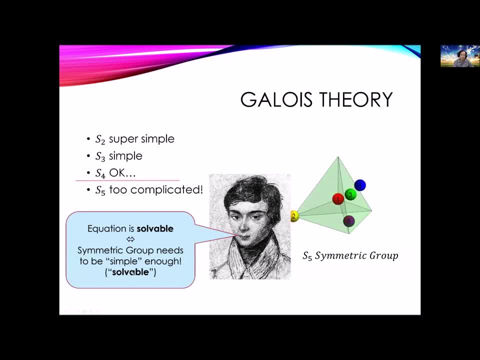 In modern term, we call this group solvable groups, which you probably will learn it in 3.1.3.1. 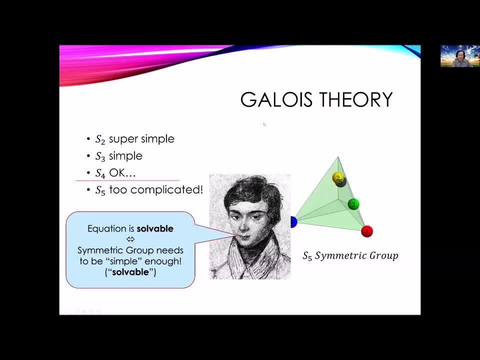 Otherwise you will never have a chance to learn it, I guess. I don't think 3.1.2.1 will talk about this. 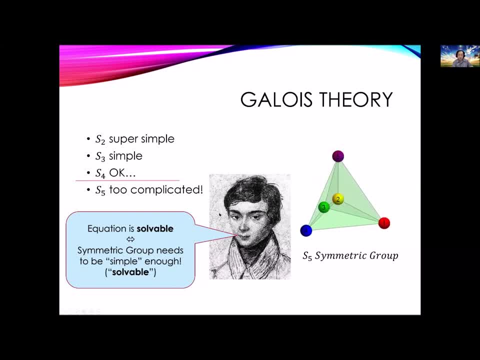 Yeah, so the equation is solvable if the corresponding group is simple enough. 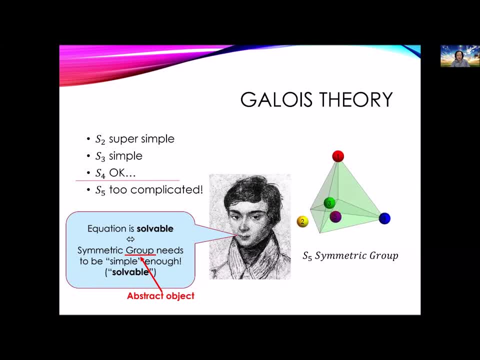 And the group he's using here is in the abstract sense. So that you are not really looking at the permutation of objects, but in an abstract setting. 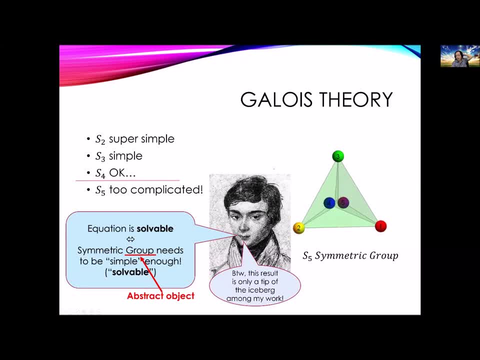 And this is only a tip of the iceberg of Garval's theory. Because I mean, Garval's theory always also related to fields and many other things. 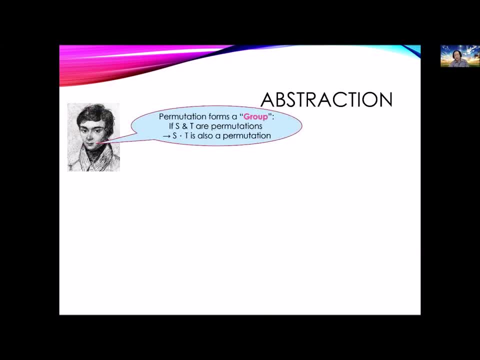 So the main observation of why, what is abstract setting is that if you have two permutations, for example, if you have this S, which is permuting two balls, and another permutation, which is permuting the three balls in a counterclockwise way, then you can compose the two. You can first apply S and then apply T like this. 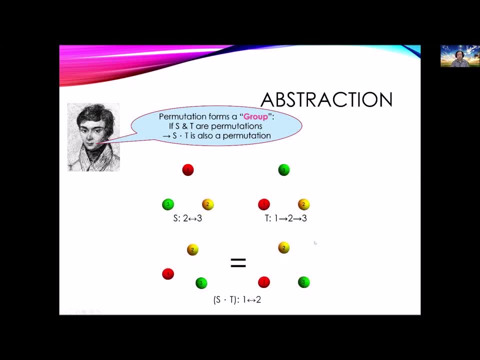 And this of course is another permutation, which is the same as just permuting one and two, right? 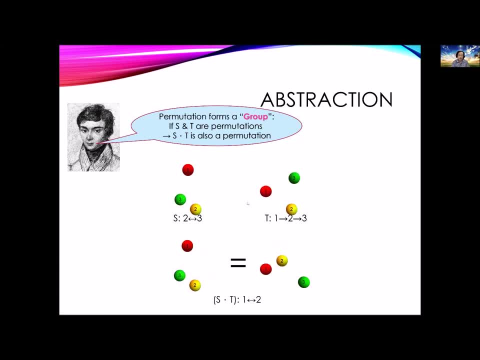 If you can compare the both sides. So permutation is closed under product in this sense. 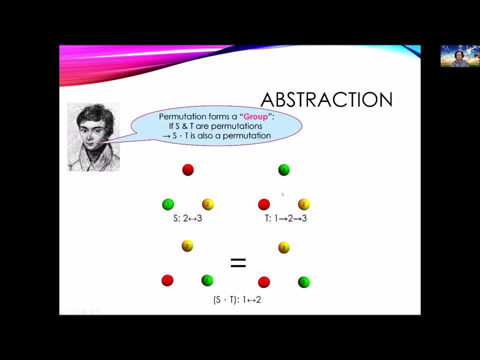 So if you have two permutations, then if you work with one followed by the other, it is still another permutation. 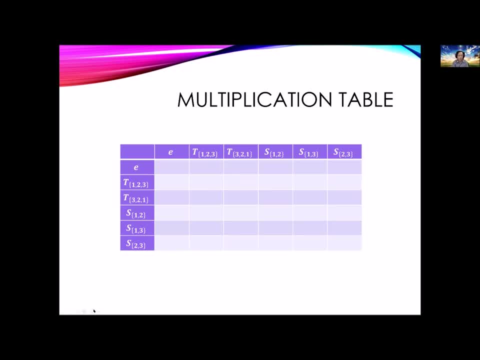 So you can make some kind of multiplication table. So for example, E is the thing that you don't do anything. 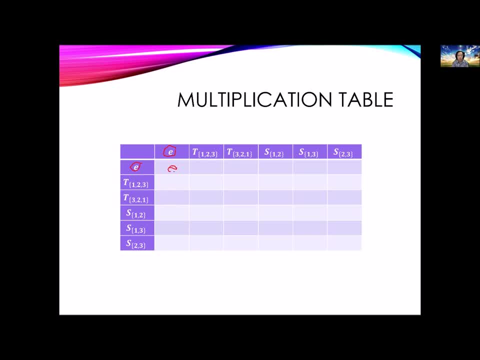 So if you don't do anything both times, then of course you don't do anything. 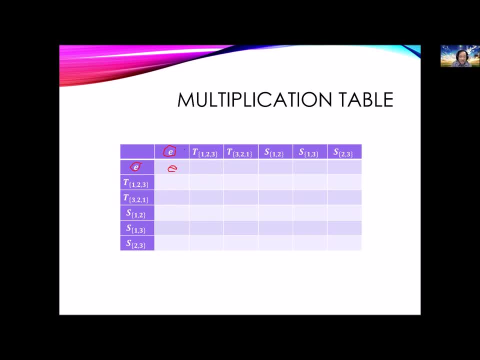 By the way, I cannot write with my mouse, so. And if you, and you think about it, 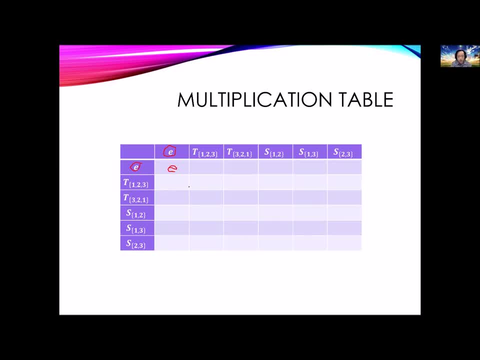 if you do a counterclockwise rotation permuting one, two, three, and then do another counterclockwise rotation again, what you'll really get, oops. Can I erase? What you really get will be T three, two, one, right? 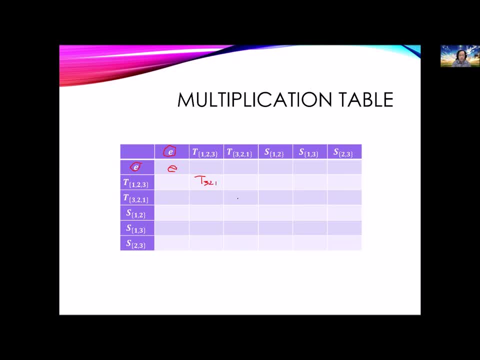 The one that is clockwise rotate and so on. 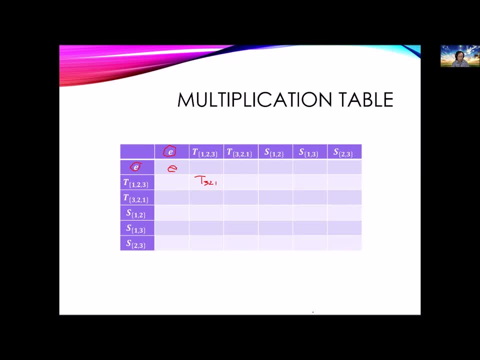 So you can fill up this table pretty quickly and easily. 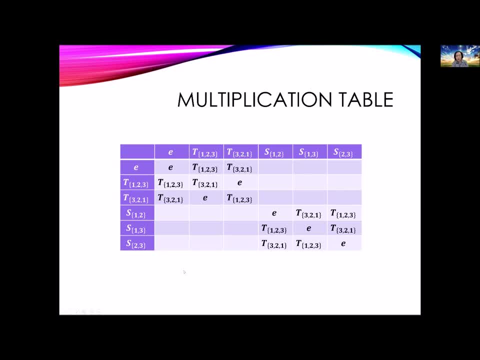 Yeah, so you can fill up this multiplication table. 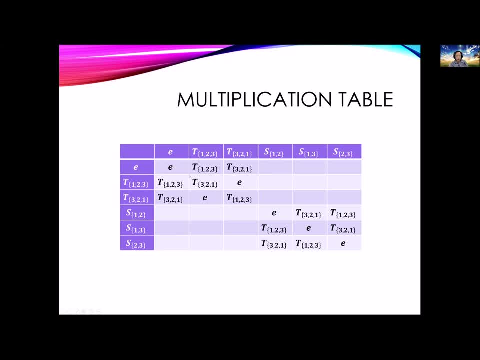 And you can see that in this way. So counterclockwise and counterclockwise, will give you clockwise. Clockwise, clockwise will give you counterclockwise and so on. And you also see, for example, that if you permute one, two and one, three, you'll really get a clockwise permutation and so on. 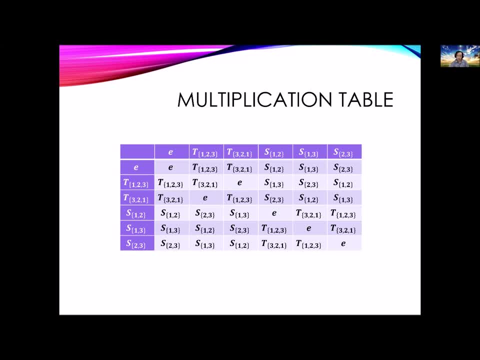 So you kind of play this game like a Sudoku. Really it's really like Sudoku. 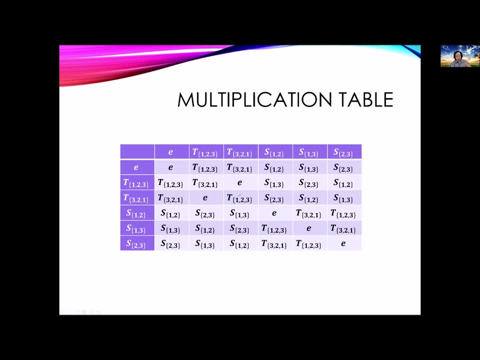 And you can create the whole table out of just observing how you permute the balls. So the example, we have just seen this, so, so, so. 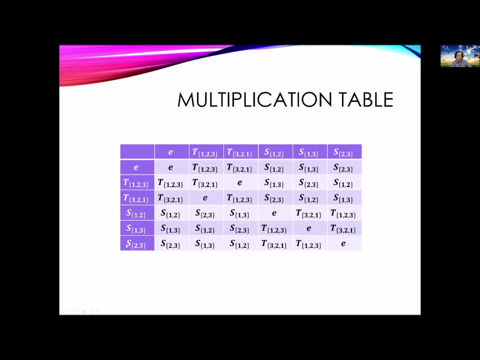 we have just seen, if we permutate, yeah, I mean, here, if we permute two, three, and then we do a rotation, we'll get the result that is permuted by one, two, for example. But this is still a picture where we have the balls, the one, two, three balls in our mind. But of course, we can just give them a new symbol. For example, I can just call this T, yeah, I can just call the rotation T and the clockwise rotation T inverse, so that when you do a rotation and then clockwise rotation and then counterclockwise rotation, you get back nothing, you get back E. And for example, when you do a permutation, flipping 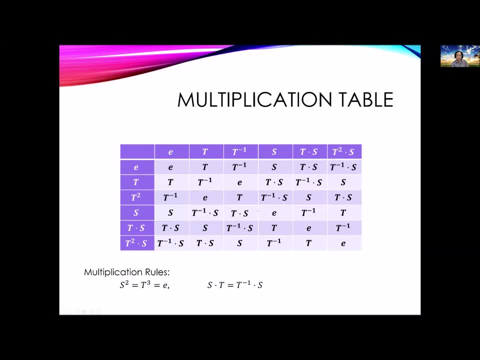 two balls, and then followed by a rotation, you will get another permutation. That would be this one, yes, something like that. 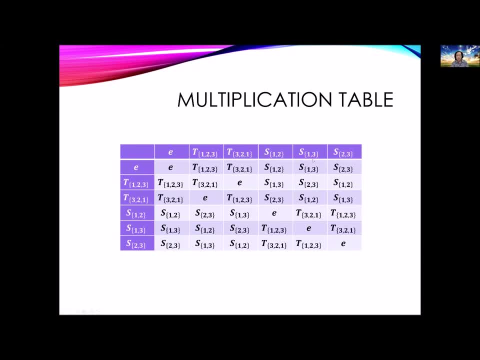 So you can, yeah, you can do that. You can represent the previous table, these tables, using just a single T and S, and represent 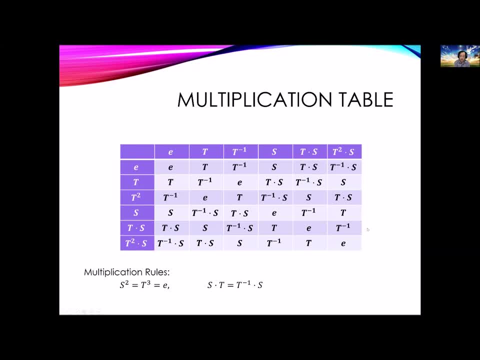 all other stuff using the abstract symbols. So now we have the groups defined in an abstract setting. We don't have the permutations in mind anymore. But instead, we have multiplication rules. For example, S, which represent flipping two balls, has to go back to itself if we apply two times. And rotation, it has to go back to itself if you apply three times, and so on. And you can also think about if you flip two balls and do a counterclockwise rotation, will be the same as first doing the clockwise rotation and then flipping that two balls. 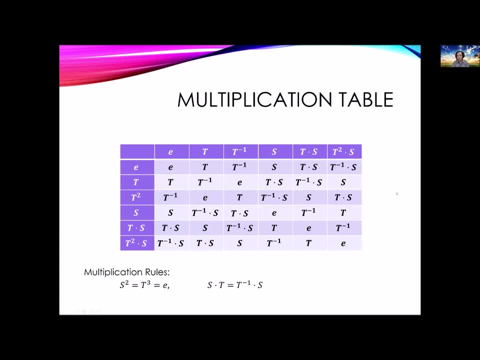 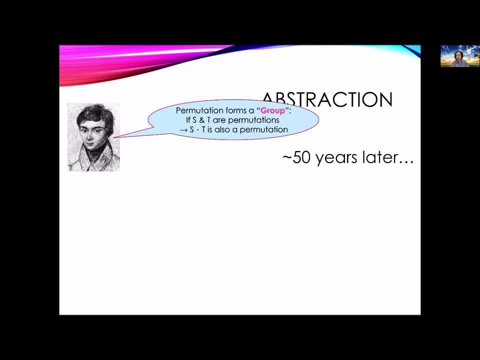 So this is a very elementary observation of a symmetry group. So it is his idea that we should study abstract objects instead of the actual equation to solve the main problem. Okay. 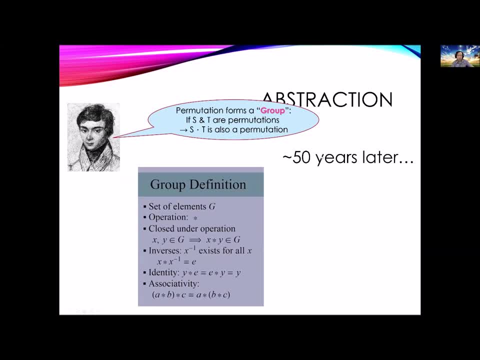 And after 50 years, different people have worked on the axiomatic definition of groups. And finally, they came up with a set of rules to define what should be a group. So a group should be a set that has an operation so that you can compose the two operations. So you should think about it as some kind of permutation. So if you have two permutations, then you should compose it to get a new permutation. And for each permutation, you should have an identity, which does nothing. And there's also an inverse, so to undo what you are doing. 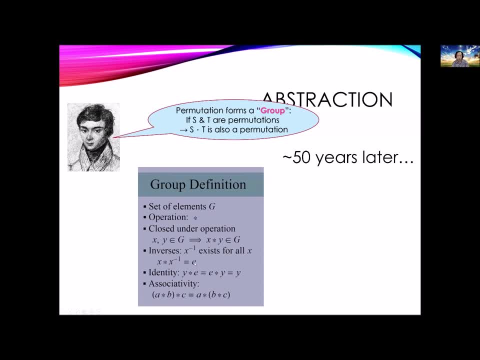 So if you are rotating, then you can rotate in the other direction to go back to the identity. 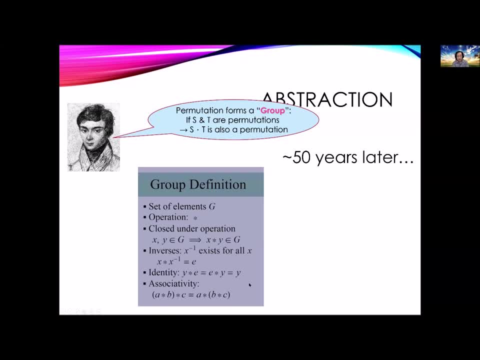 And finally, associativity is also a very natural condition, because remember permutation is really mapping a set of numbers to a set of numbers. It's like a function from numbers to numbers, changing the numbers, but still a function. Okay. It's like a function from numbers to numbers, changing the numbers, but still a function, but still a function. 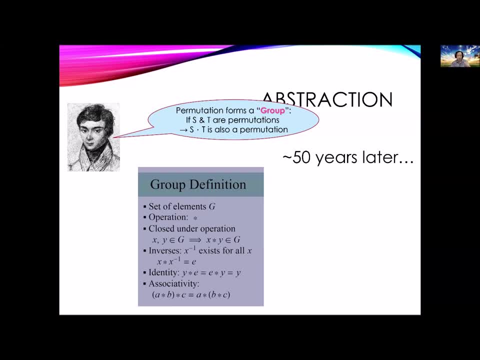 And we all know that composition of functions are associative. f of g of h is f of g of h. So this associativity for group is a very natural condition. So there are basically three things. You have identity, you have inverse, and you have associativity. Or in layman term, you can multiply and you can divide in a group. 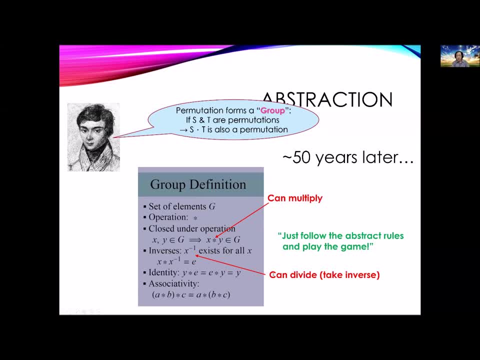 So in modern mathematics, the philosophy now is that starting from these axioms or these abstract rules, you just follow them and play the game by trying to derive as many results as possible, just starting from these axiomatic rules. 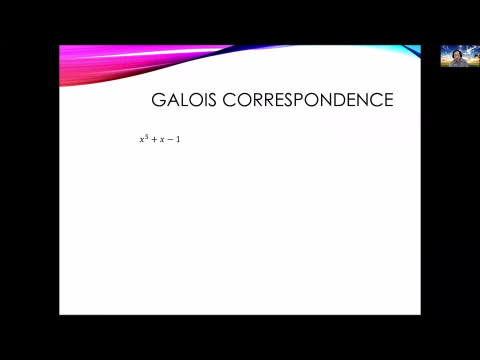 So now the question, one other question is, Galois says that quintic equations cannot be solved, but what precisely does it mean? So does it mean that every quintic equation cannot be solved? Well, I mean, that definitely is not the case. For example, this quintic can be factorized. 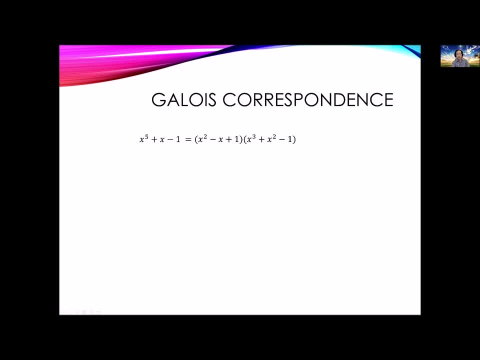 And if you can factorize, then of course this can be solved, because you can solve both factors separately, right? So Galois's correspondence means there is a correspondence between the symmetric group of the polynomials and the structure of the field extension from the roots. So we have seen that the quadratic corresponds to s2, which is just like a flipping two balls, so it's very simple. And the cubic will correspond to s3, flipping three balls. And we have seen that there's some kind of 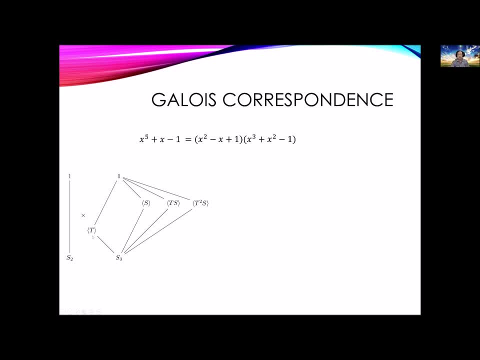 of subgroup structure for example you can only focus on rotations and if you do rotations then you can always only get rotations you cannot get flipping from rotations alone and you can also 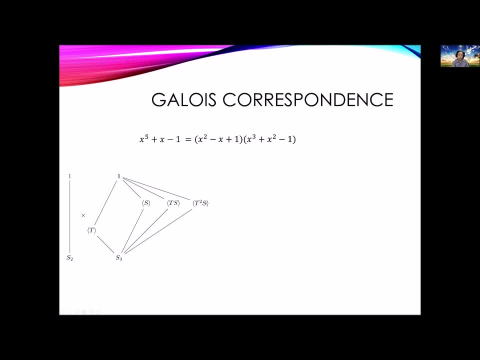 do flipping alone so this is flipping one two flipping two three flipping one three and this 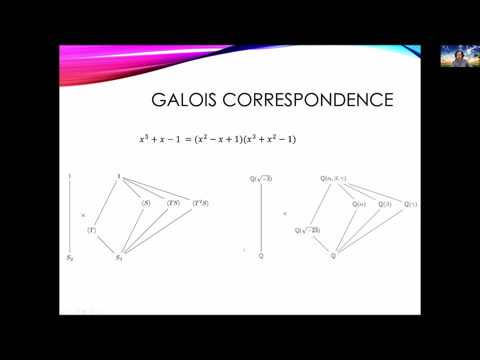 form kind of substructure called a subgroup and this will correspond to the roots of these polynomials so for example with the quadratic you can see that it can be solved by including 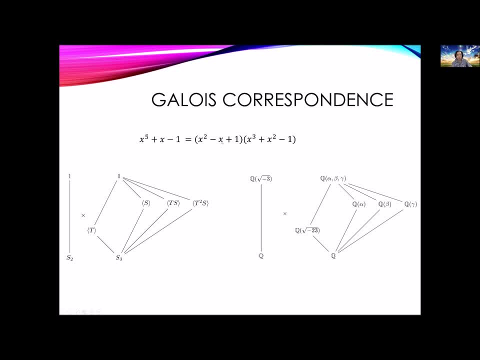 negative square root three square root negative three into your numbers and for the cubic you can solve the equation by introducing square root negative 23 and some auxiliary roots 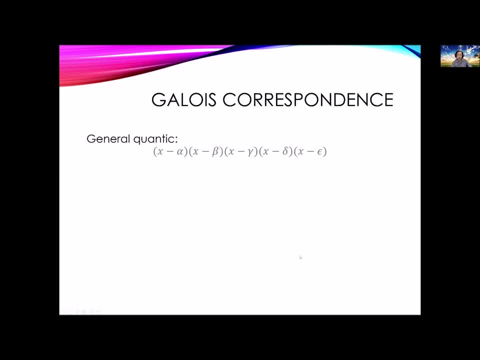 and so the point is that for general quintic where you have five roots the symmetric group is s5 the real s5 and the symmetric group is the real s5 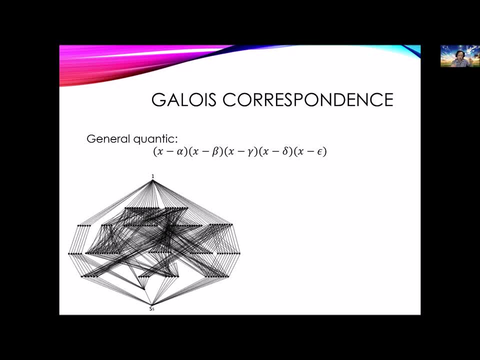 and it looks something like this which is true complicated and you still have the correspondence between the root extension the field extension using the roots of this polynomial with the base 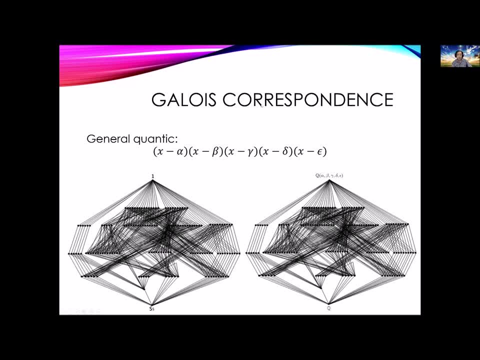 field and this is what gawao actually did is to find a correspondence between symmetric groups of your polynomial and some field extension using the roots of your polynomial and so he successfully 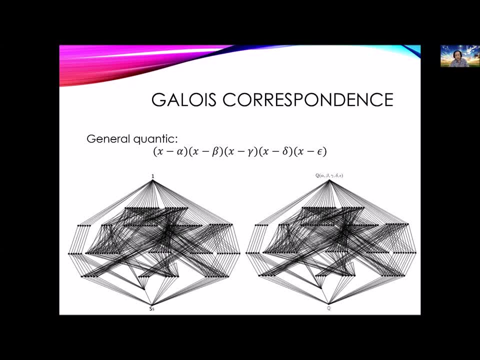 turned a concrete problem of solving equations into studying abstract structures and substructure substructure of some mathematical objects called groups 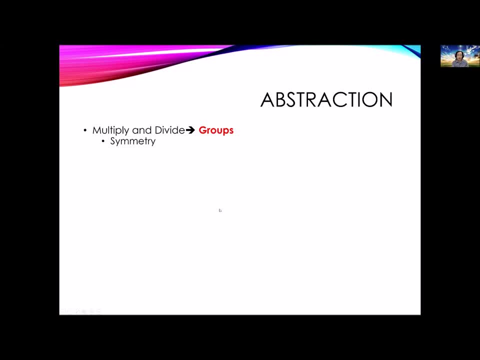 so as i mentioned groups means multiply you can multiply and divide and this leads to symmetry but of course you can also add more rules like if you allow addition and subtraction and multiplication together just like integers for example then what we get is a structure called ring 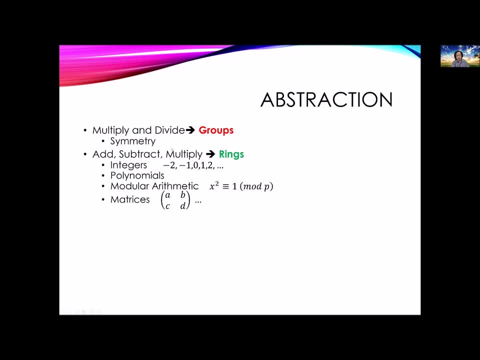 and there are many examples of rings like integers like that you can add subtract and multiply polynomials of course you can add subtract multiply and some modular arithmetic and matrix 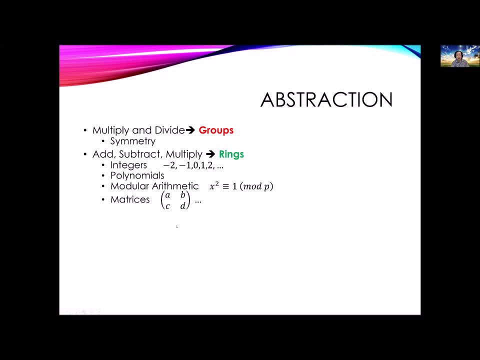 also matrix you can add a matrix subtract matrix multiply matrix but sometimes you may not be able to divide a matrix by taking inverse if you want to divide something then the structure will be 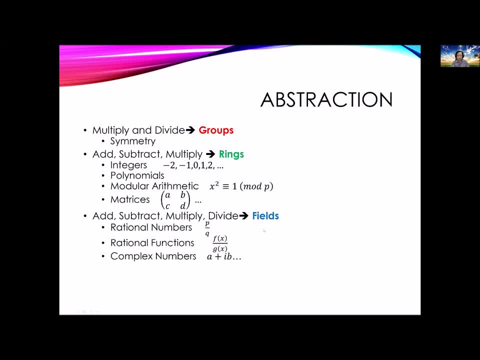 called a field so if you include division then for example instead of integers you'll have rationality then you'll have rational numbers and if instead of polynomials you have rational functions and there are many other examples like complex numbers you can definitely divide complex numbers so the 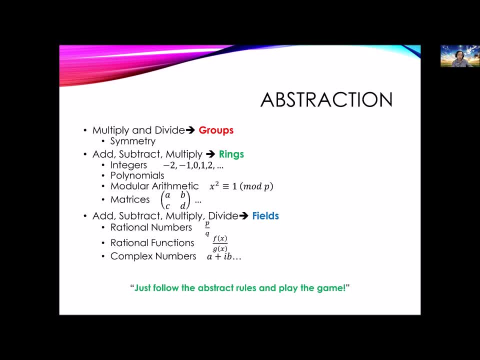 main philosophy as mentioned before is just start by abstract rules and play with the game so don't be scared about extra algebra it is really just doing arithmetic but in a more general sense 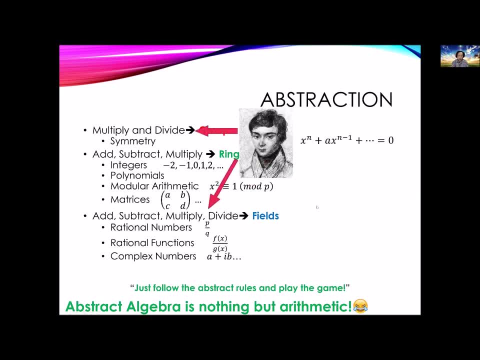 so groups and fields are developed purely because of Galois theory to solve n degree solvability of degree n polynomials. 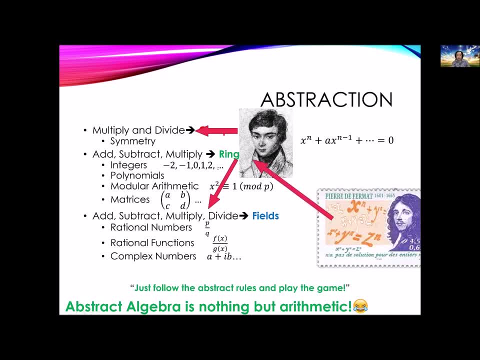 While ring theory actually has a different history. So ring theory was mostly developed because of Fermat's last theorem. 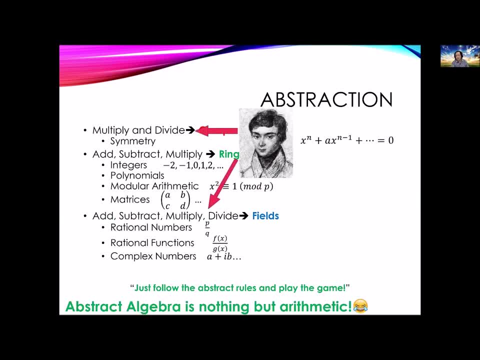 You know, this film has been troubled mathematicians for 350 years until it is solved by Andrew Wiles in 1994. 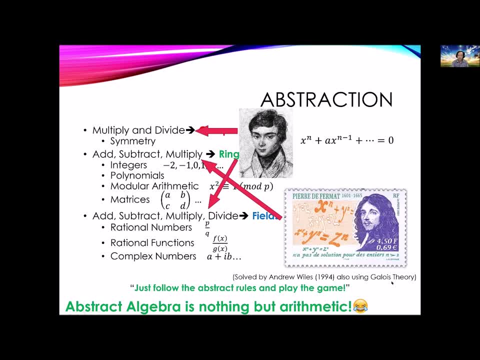 And his proof also use a bit of Galois theory. So, yeah, I probably will not have time to give another talk on the development of ring theory, but the main philosophy kind of get together now 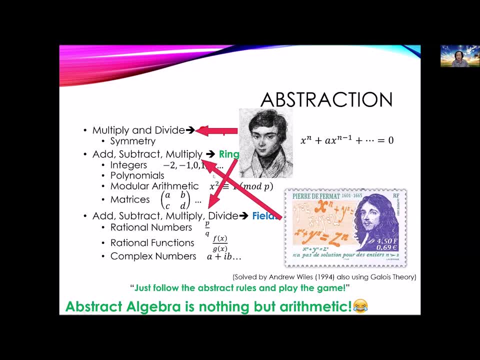 that to study modern mathematics, we have to do abstraction. And yeah, also, we also have a first day cover for Galois. 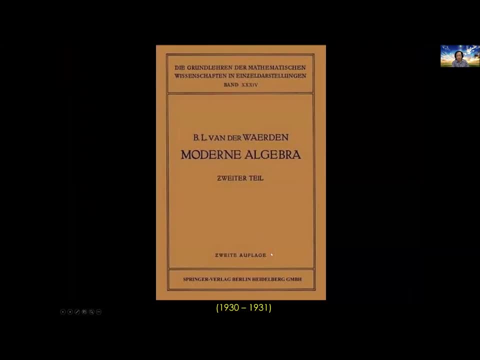 So finally, the first book on modern algebra that really deals with this asymmetric definitions and abstraction is this book by van der Weerden. 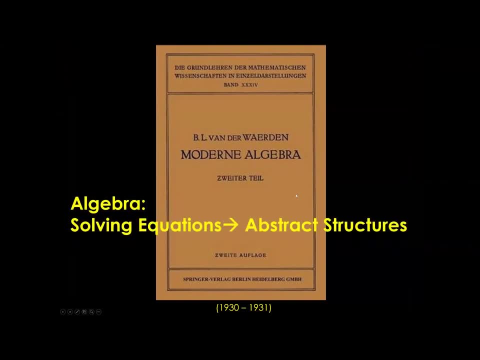 It was published in 1931 in 1930. And from that on algebra turns from solving equations into studying abstract structure. And this is also the beginning of the asymmetric approach to mathematics.